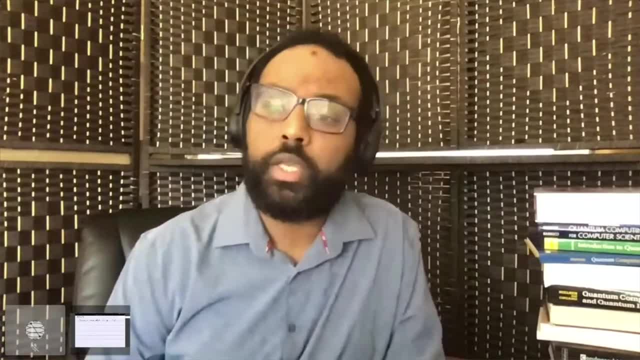 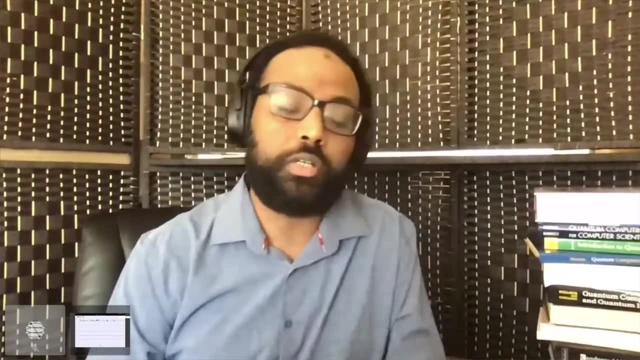 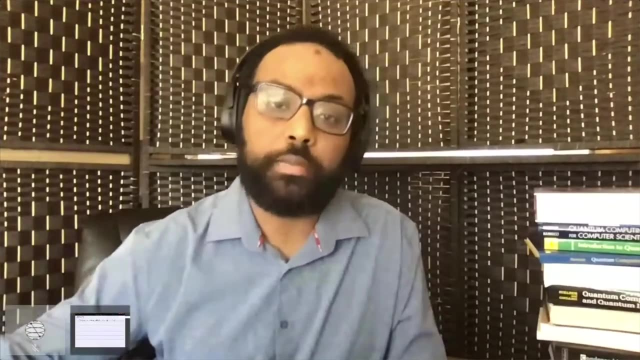 focused on building out quantum programs. So you're about to transition from the starting point, which is where you are learning about quantum concepts in general and how to work with quantum algorithms, into a slightly more advanced concept now, which is building quantum programs. 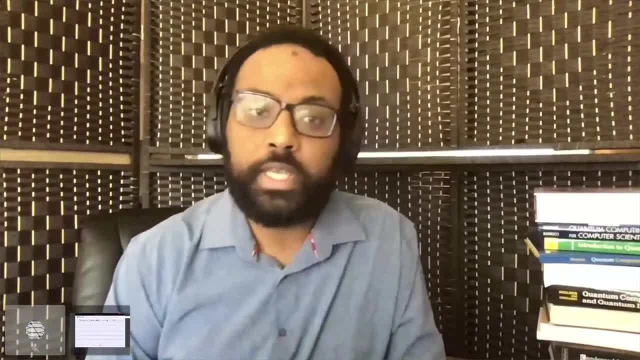 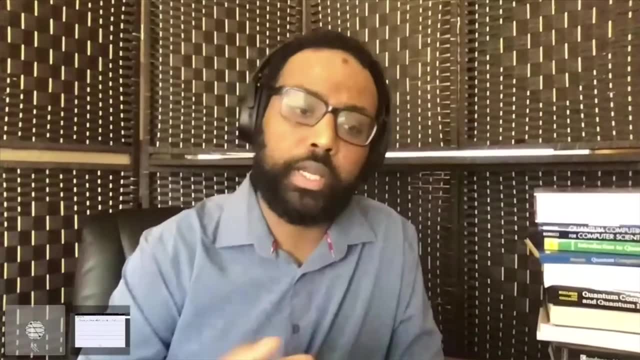 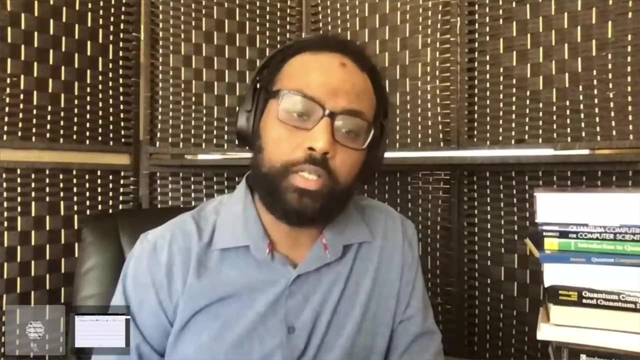 using quantum algorithms. So today will be your first exercise. The program that we're going to be building out is called Shor's Algorithm and it's a factoring program, But what I would like to do is just give you an overview of what we've done so far. do a quick review. 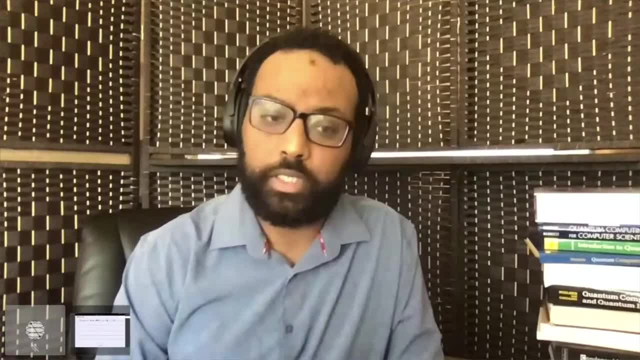 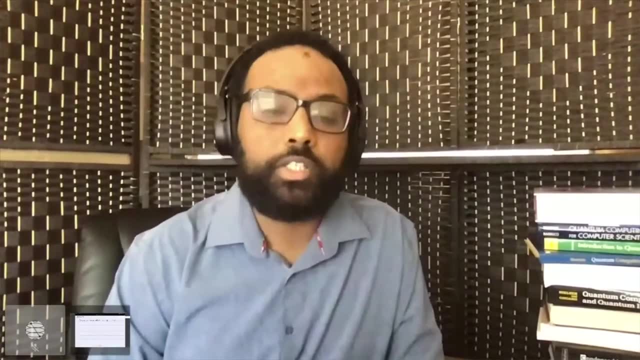 and then show you the preliminary concepts involved in Shor's Algorithm. So we're going to learn about Shor's Algorithm in two lectures. The first lecture is going to be today's lecture and we'll be talking about components of Shor's Algorithm called 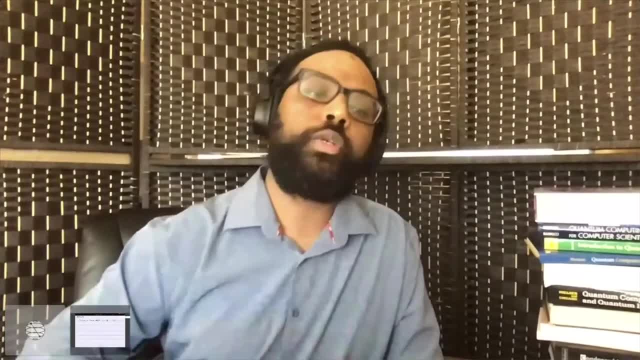 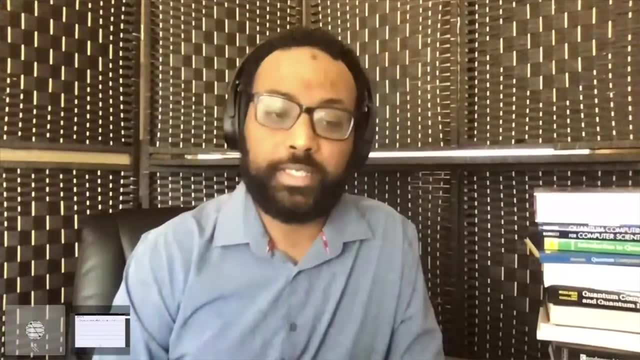 the quantum Fourier transform, And I'll also show you a related concept called quantum phase estimation, which uses quantum Fourier transform. In tomorrow's lecture you'll see the exciting part where we put all of these learnings together and build out Shor's Algorithm. 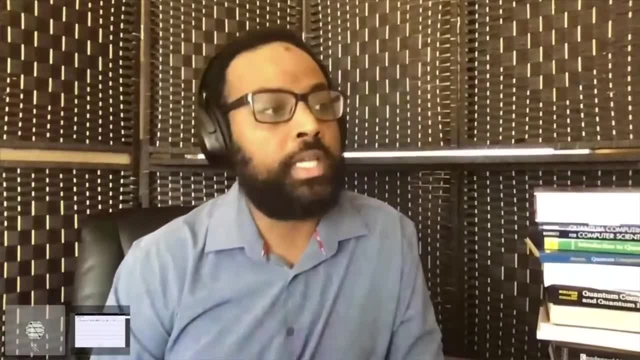 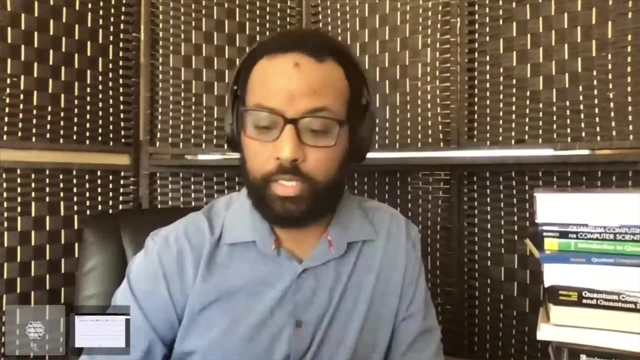 Now Shor's Algorithm- I keep repeating this name just to give you a quick introduction- is one of the crown jewels of this field. It's one of the algorithms that, as soon as the research results came out, started a lot of excitement within this field. 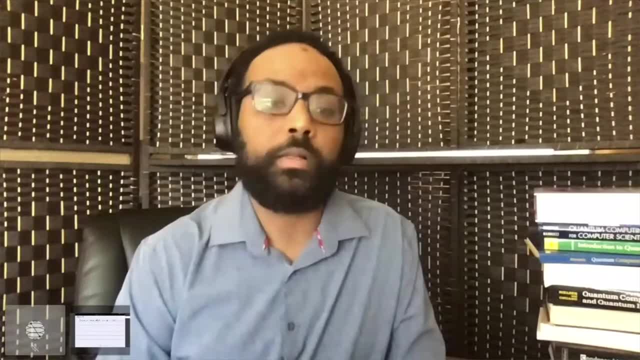 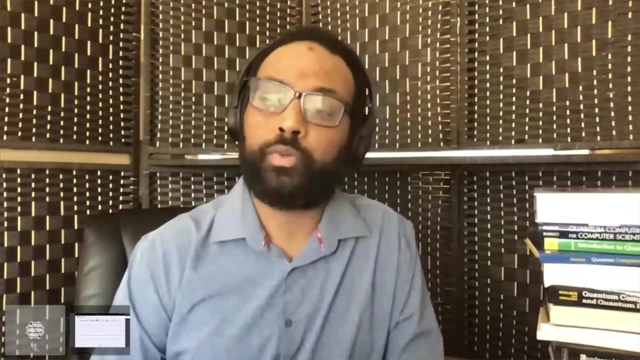 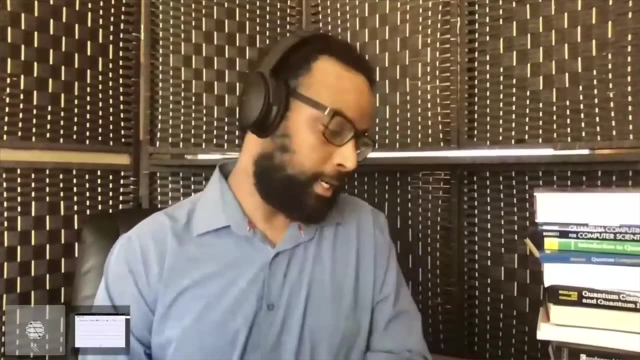 So I really want to show you the core of Shor's Algorithm in detail, but what that will require is going through the preliminary concepts today, and then tomorrow we'll go through Shor's Algorithm by putting all of these things together. All right, so I'll begin by sharing my writing pad here and turn off my video. 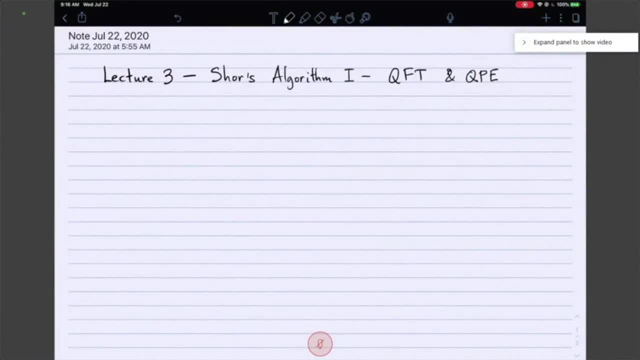 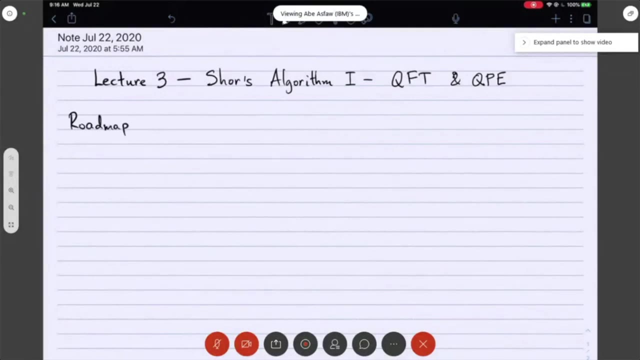 And then I'll start discussing with you about Shor's Algorithm. So let's do a quick roadmap. So where have we gone so far and what are we going to learn today? So I'm going to write down roadmap and review some very quick concepts that we've learned. 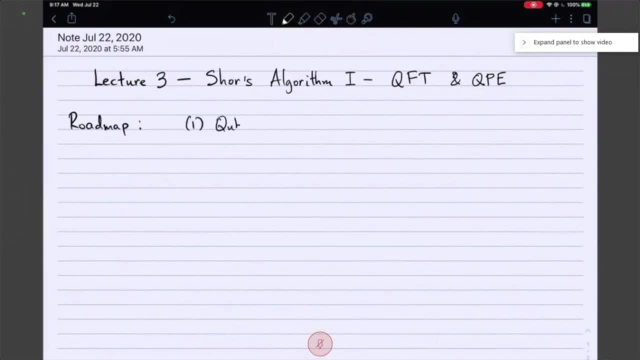 So what did we learn? We talked about qubits and quantum states in the very first lecture. So what does this mean? We talked about qubits and quantum states, so we learned things like the zero state, which is this kind of notation that you've seen in your lectures. 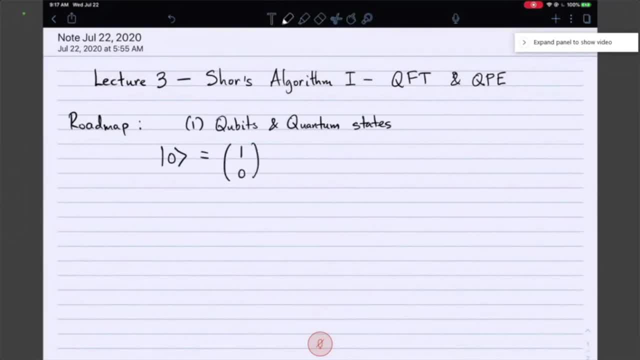 is really just a vector that looks like this. It's just one and zero. The one state is really just something that looks like this, And you also went through several gates that you could use to manipulate these quantum states. In particular, you went through things like the Hadamard gates, which, if you remember, look something like this: 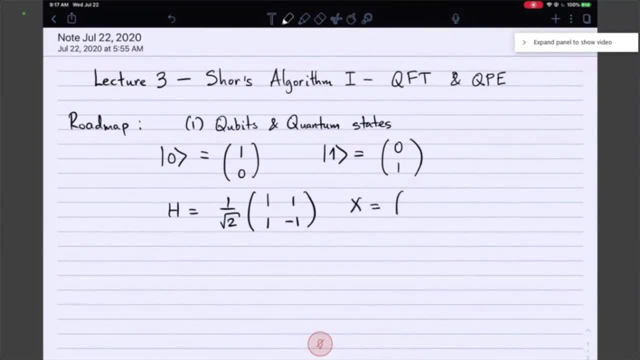 And we also saw, maybe the X gate, if you recall, which looks like this. Now, all of these concepts are very important to learn and all of them are quite useful for you to keep in mind and maybe even memorize. But what the fundamental concepts? 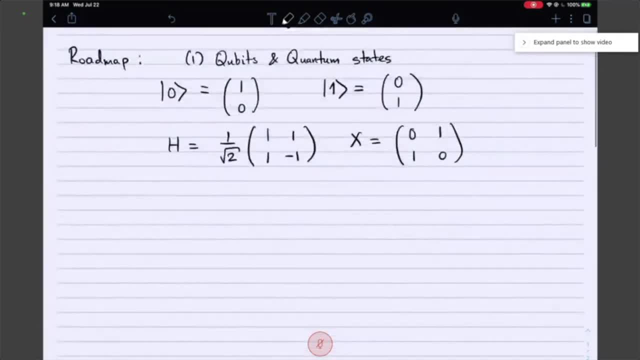 are that you learned centered around manipulating the quantum states, or the wave functions, which we wrote down generally as psi, to be of the form a0 plus b1.. What does this mean? You learned about how to measure specific parts of the state. So for. 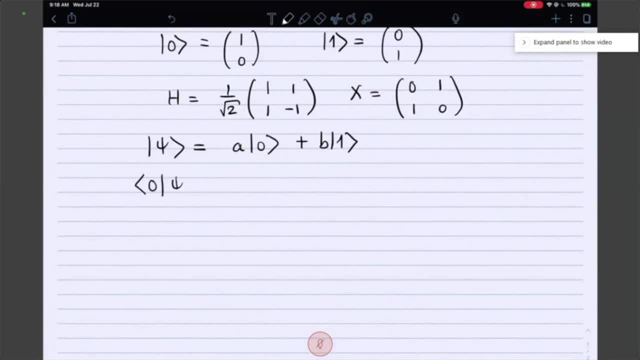 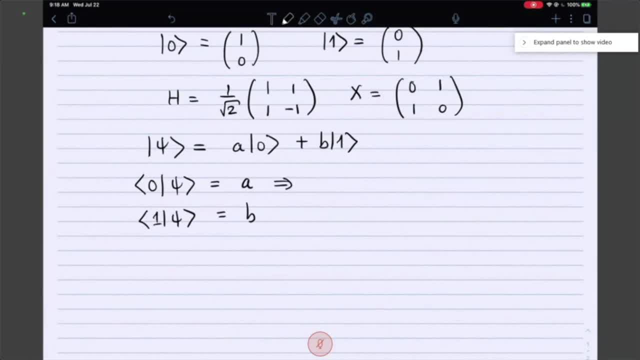 And more generally what that means is, if you were to measure psi, the probability of measuring zero is the norm of a square. So if a is a complex number, you're taking the magnitude of that complex number, And if you're measuring psi, the probability of measuring one is equal to. 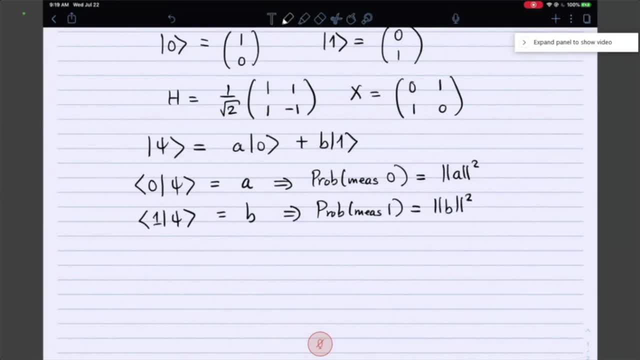 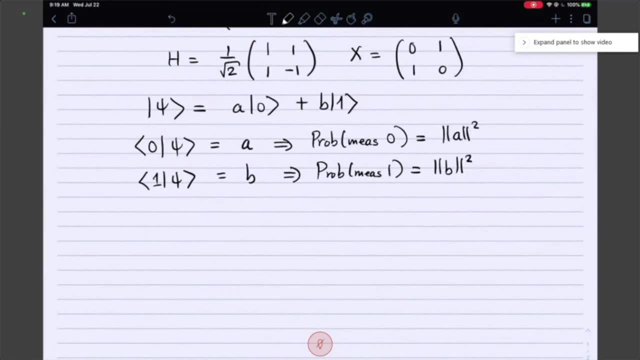 b. you're taking the magnitude of that complex number b and you're squaring it. What is the most important thing that we've learned so far? Well, if you measure this particular state, you have to get either zero or one. 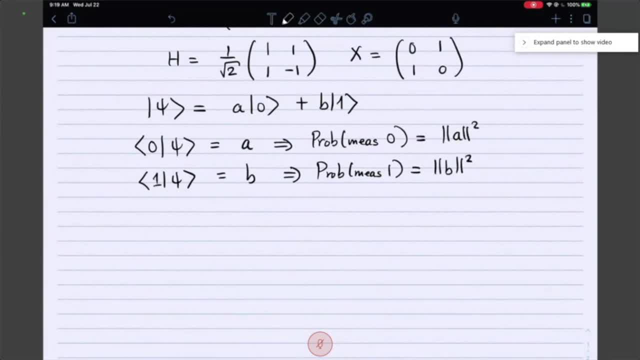 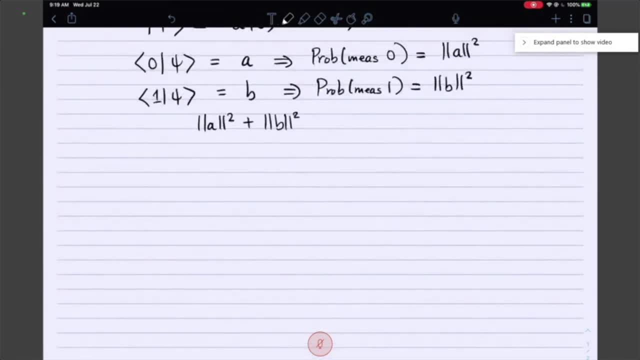 So these two probabilities have to add up to one. So we made the statement that these two norm of a square and norm of b square have to be equal to one, and this statement has two implications that I'll point out to you. So here are the two implications. So implication number one: 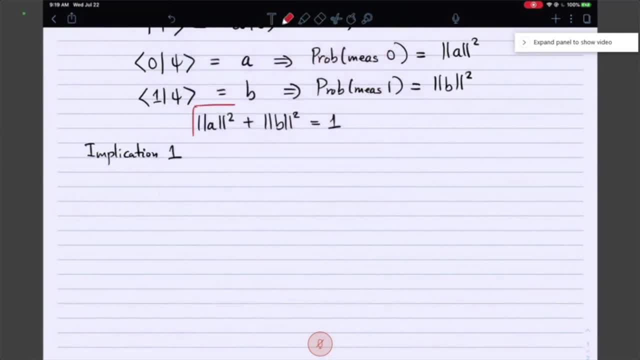 of the following statement is: operations on quantum states need to preserve the norm, And the way they preserve the norm has to be exactly equal to one, which is what we've seen. What does this mean? This is actually a very complicated sounding way of just saying. 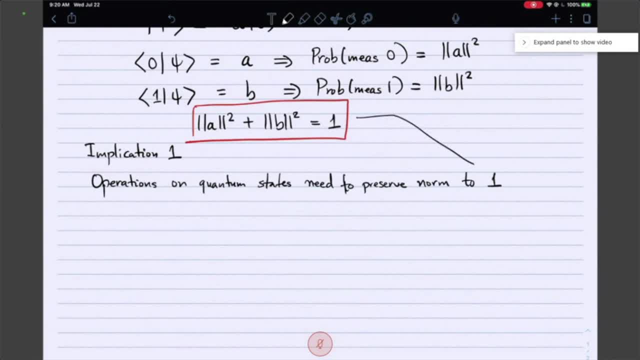 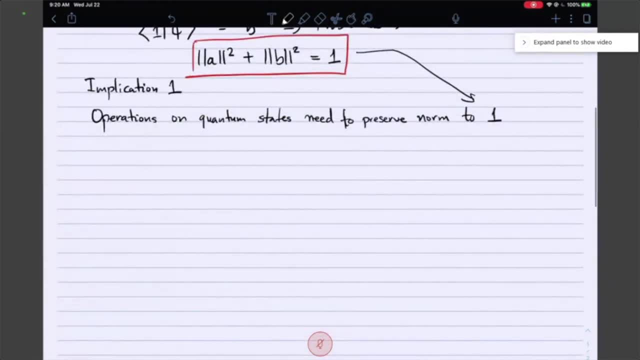 we have to be able to maintain this condition, no matter what kinds of gates we apply. Okay, so what exactly does this tell us? Well, that tells us that the kinds of operations that we can apply always have to preserve the norm, and the kinds of operations that do that are called unitary operations. So 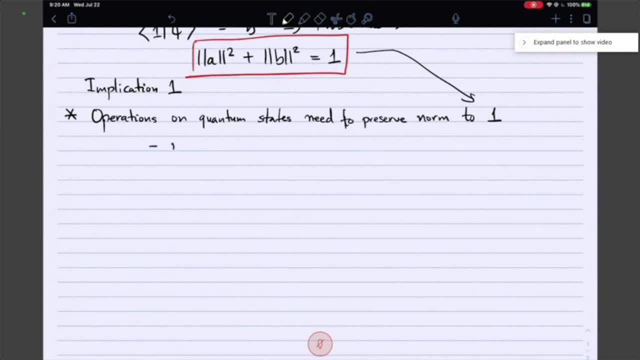 this is why the kinds of operations that we've been applying are norm-preserving, And norm-preserving matrices are commonly called unitary matrices And for those of you who have some linear algebra background, what this means is the complex conjugate, the transpose of that matrix. so U dagger is equal to U inverse. 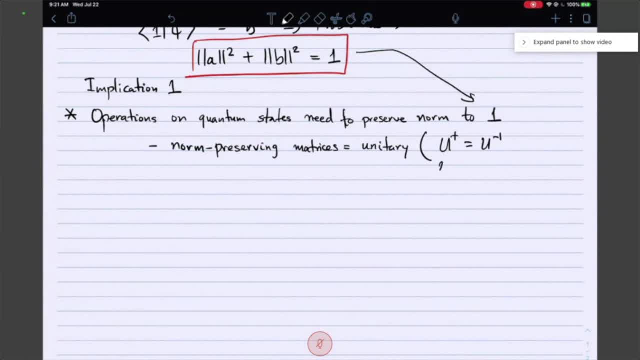 So what does that mean? If you take the dagger of that matrix and multiply that to itself, that's the same as well. You can do it in any order you want. So U dagger, U or U U dagger. At the end of the day, this is the identity matrix. So what it means is, if you apply the 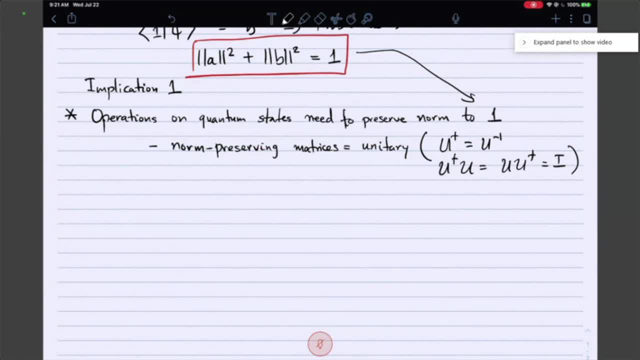 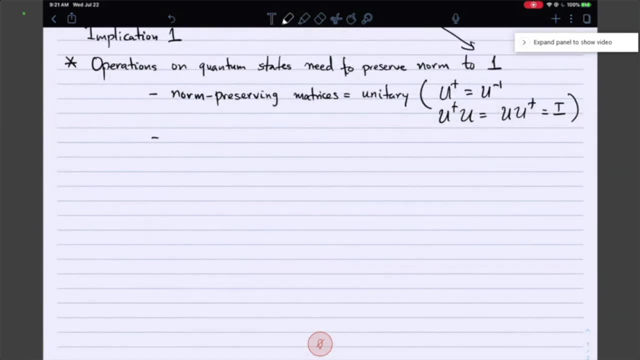 unitary operator and then its complex conjugate transpose. that should give you an identity. That's like doing nothing. Okay, so why does this work? Well, one of the key features of these unitary matrices. so if you write down any of these unitary matrices, you'll find the determinant. 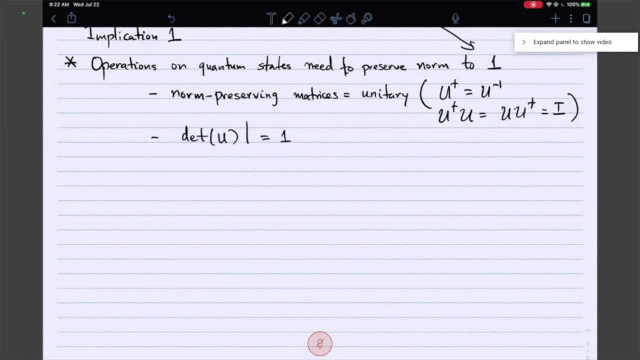 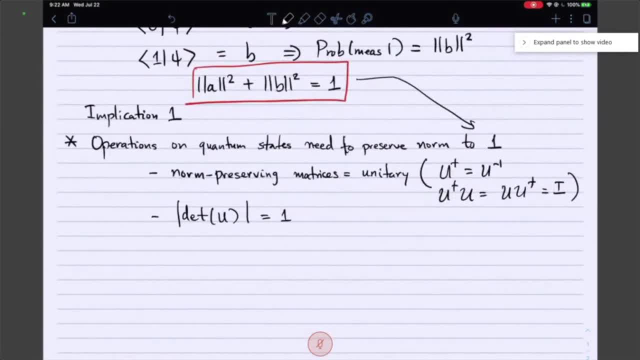 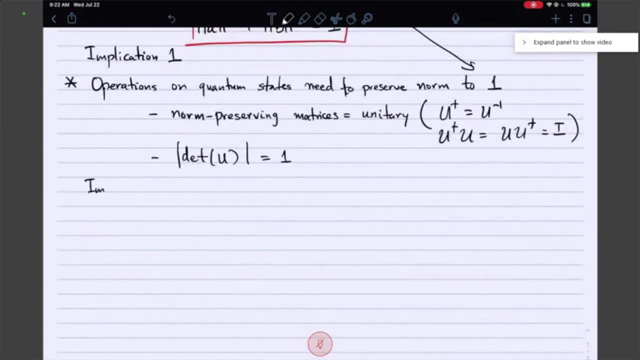 very, very, very. First implication of saying that norm of a square and norm of b square have to be equal to one. What is implication number two? Implication number two is for a single qubit. you can think of unitary gates, which are the gates that we talked. 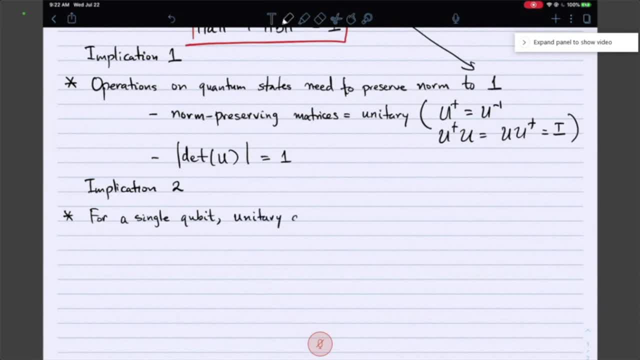 about, So that these gates are rotations on the surface of the block sphere. So why does this work? This works because the block sphere is a unit sphere, So its radius is equal to one exactly, And so you're maintaining that radius equal to one as you're rotating on that surface. 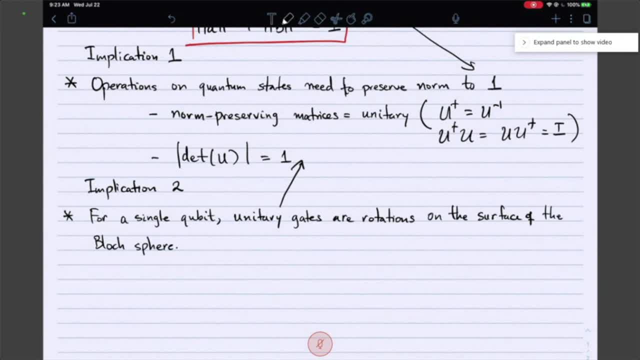 So you've seen in the first lecture that applying rotations onto these single qubit gates is exactly equivalent to applying unitary matrices onto them. Okay, So that's another important concept to keep in mind. You've seen both of these implications so far in your lectures. 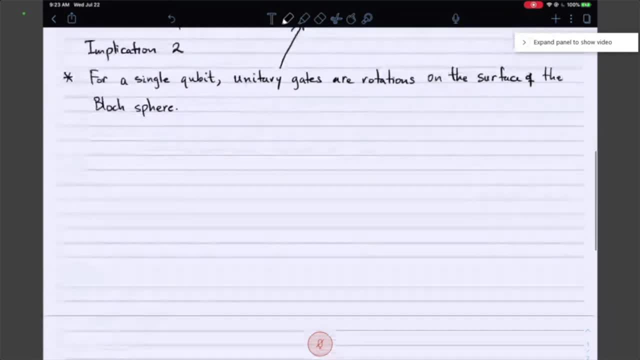 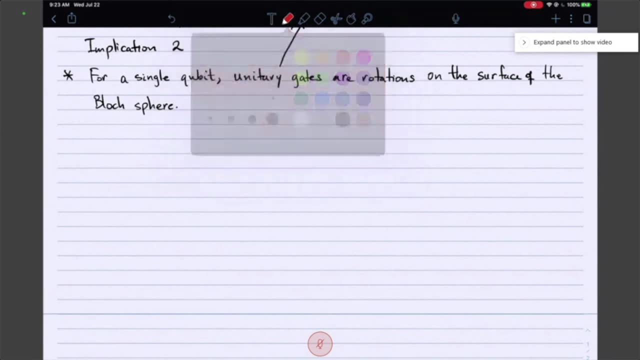 Maybe you may not have noticed. I'd like to point out to you a third implication that comes out of these, which will be important for today's lecture. So I'm going to change the color here very quickly and remind you implication number three, which is the eigenvalues and eigenvectors of unitary matrices, which are exactly the 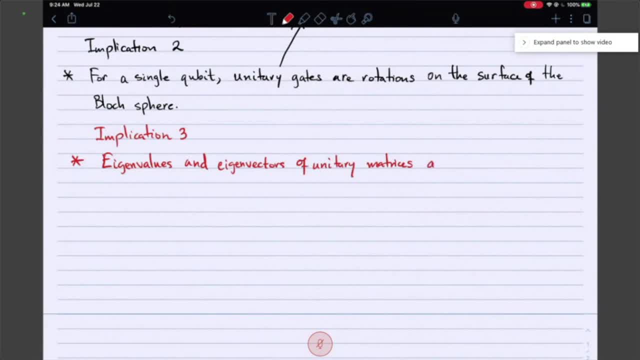 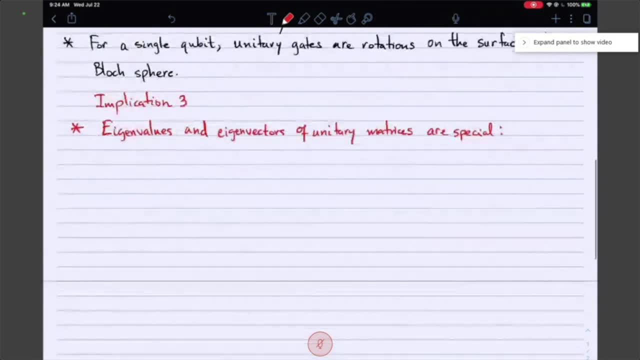 gates that we're talking about above. Okay, So the eigenvalues and eigenvectors are special. How are they special? Well, first of all, let's talk about what it means to have eigenvalues and eigenvectors. The eigenvectors of this particular unitary operator U are the vectors such that, if I 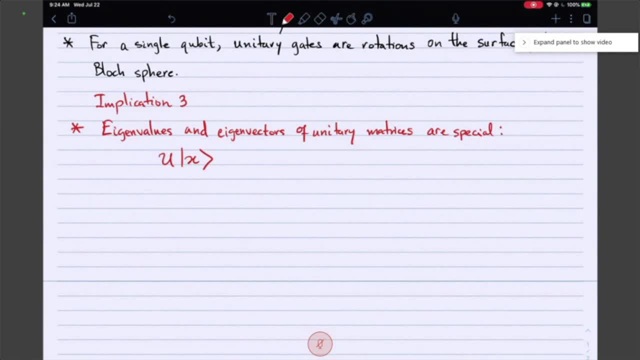 apply U on that particular state, I would get exactly that particular state with some coefficient in front of it. So let's call that lambda X. Okay, Now there are a couple of conditions I'd like to tell you, without going through the proof in a lot of detail. there are two things that you have to keep in mind. 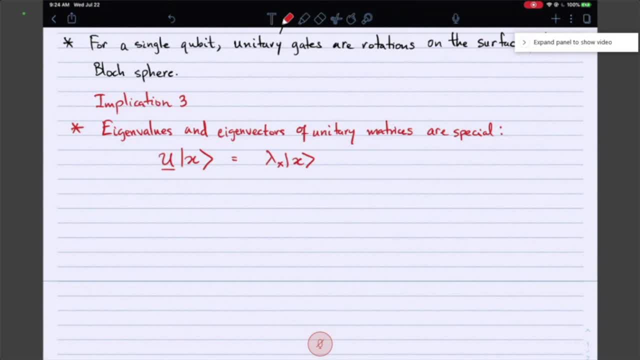 For unitary matrices, which are exactly the ones that we're dealing with, these eigenvalues. so this one is the eigenvalue and this one is the eigenvector. just as a quick refresher. the eigenvalue has to be of the form. 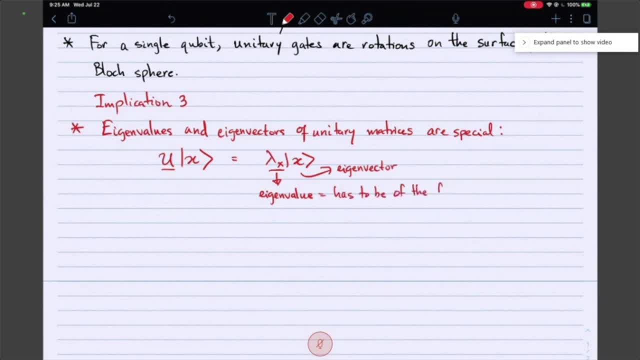 E to the I theta. So what does that mean? It has to be a complex number and a very special kind of complex number that has magnitude one and just looks like a phase on top of something. So there's a theta coefficient that comes there. 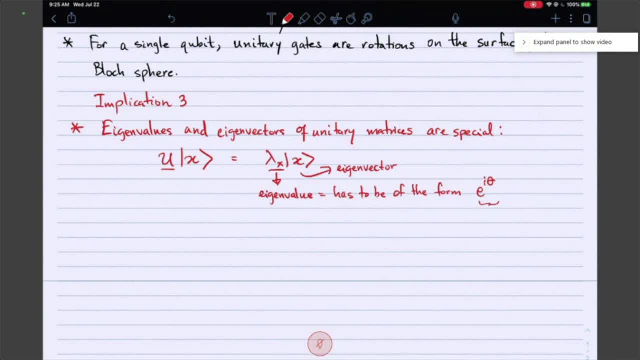 Okay, So that's a very significant statement that I'm making here. What I'm telling you is that when you apply the unitary operator, what you're doing is you're effectively applying a phase onto its eigenvectors. Okay, So that's the most important part. 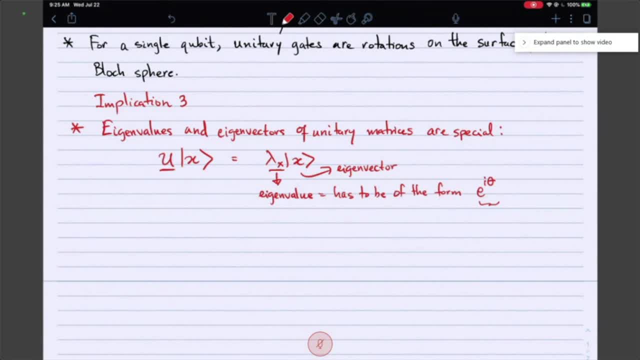 And, at the end of the day, all this is telling you. it's just a very fancy way of saying all the unitary matrix is doing is rotating. that particular is adding a global phase onto that particular, onto that particular eigenvector. 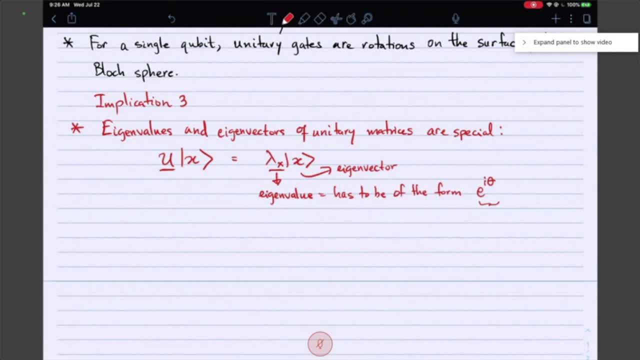 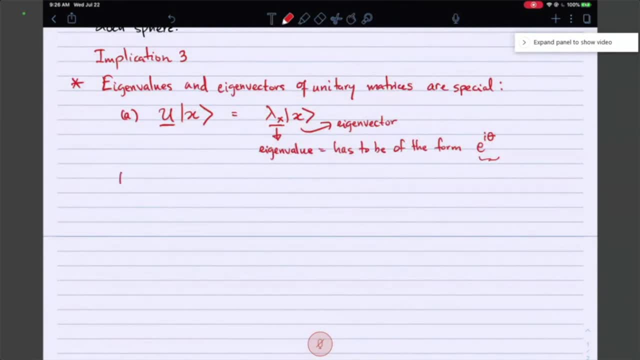 Okay, The second thing I want to point out to you. so this is something special about the type of the eigenvalue. The second thing I want to point out to you is that if there are two eigenvalues, so let's call them Lambda X and Lambda Y, if they're not equal to Y, if they're not equal to each. 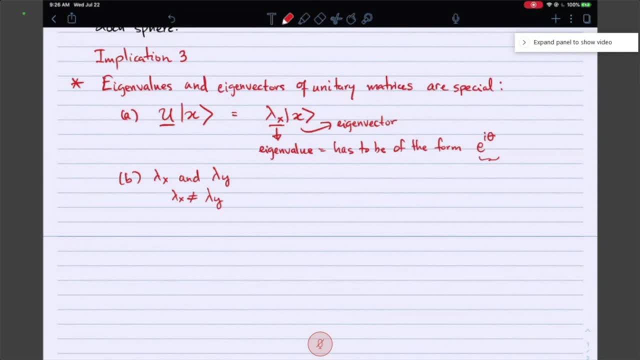 other, excuse me, then we can say something very profound. What we can say is: if Lambda X is not equal to Lambda Y, Okay, Okay. Okay, Then the corresponding eigenvectors, let's call them X and Y, are orthogonal. 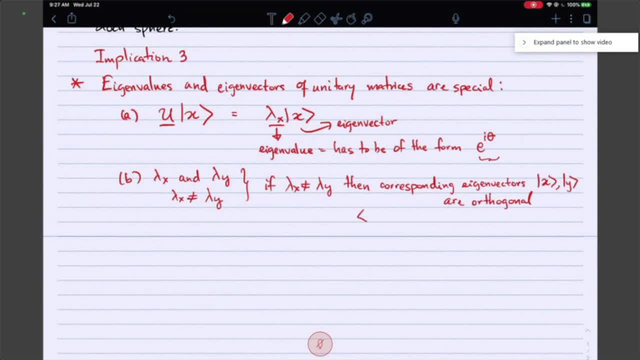 What does that mean? That means if you take the dot product of X and Y, it has to be exactly equal to zero, And this is another very important thing to keep in mind. So, in principle, you've already learned about all of this. 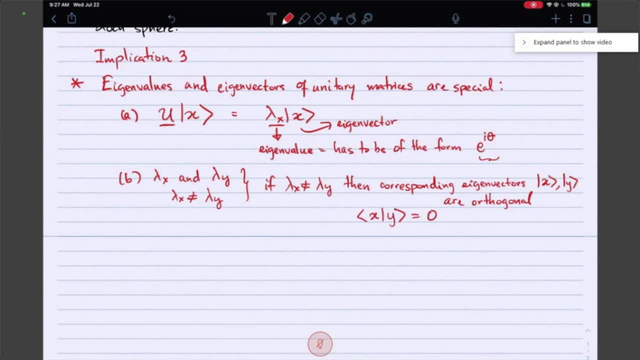 It may not have been apparent as you're going through the material, but it's good to highlight these points because I think they'll be useful in the rest of the lecture. So again, quick, quick review of what we just did. We said the unitary matrices have special conditions on their eigenvalues and eigenvectors. 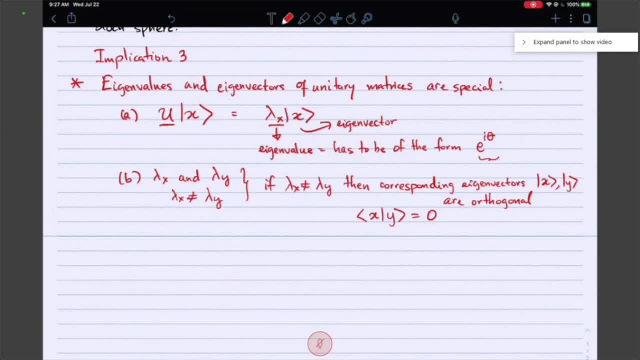 The eigenvalues I told you have to be of a special form which looks like this: E to the I theta. And we made also a statement about the eigenvectors. Given two different eigenvalues corresponding to two different eigenvectors, I know that those two different eigenvectors have to be orthogonal. 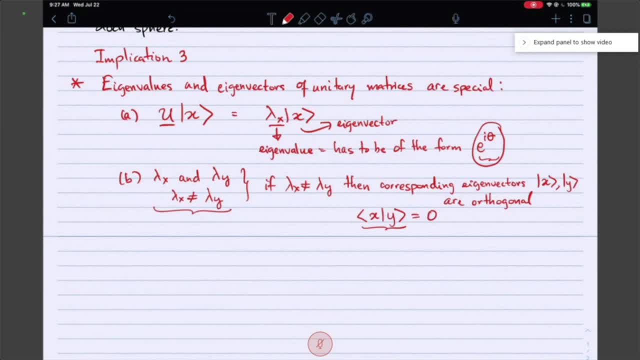 And this is something that we'll learn as we go. So just as I'm going through this material, I'm watching the discussion in the chat very quickly and seeing people asking questions like: what is the difference between a unitary and a Hermitian matrix? 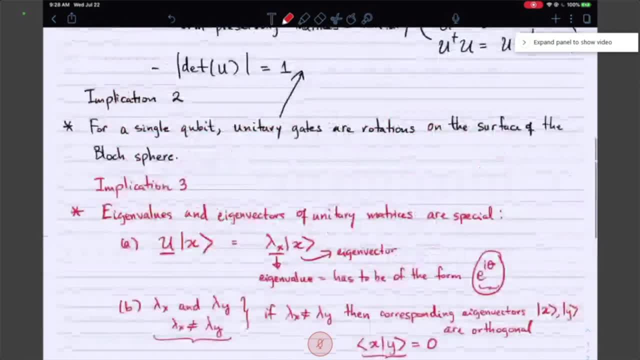 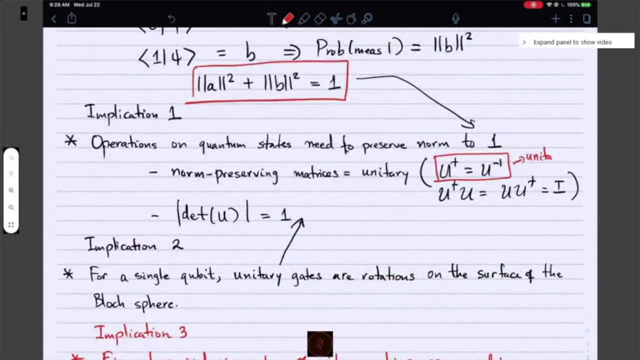 I'd like to remind you again. So unitary matrices are the kinds where U dagger is U inverse. This is unitary. Hermitian means U dagger is equal to exactly U. Notice the difference: U dagger is U inverse for unitary and U dagger is U for Hermitian. 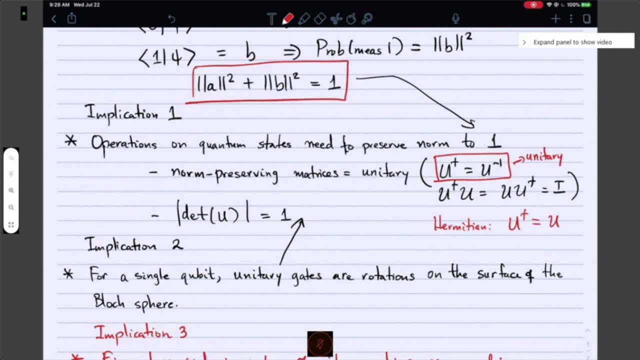 I hope that clarifies the difference between those two kinds of matrices. They're both very important And they're actually very, very important uses generally in quantum physics. But I think for this particular context today, I'd like to focus on unitary matrices because I think you'll see some key things coming out of them. 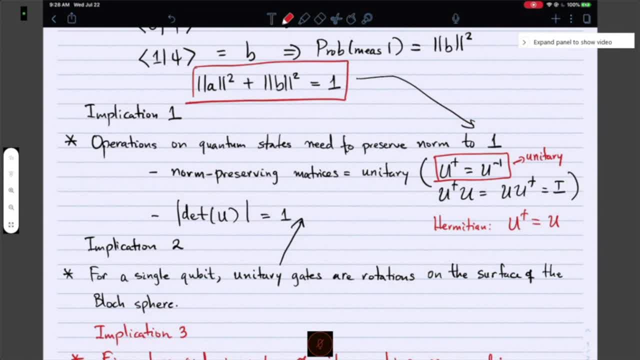 And in fact later on, as we're dealing with quantum phase estimation, you'll see that unitary and Hermitian matrices are actually very closely related. There's a very close relationship between the two, All right, So I hope that has been. 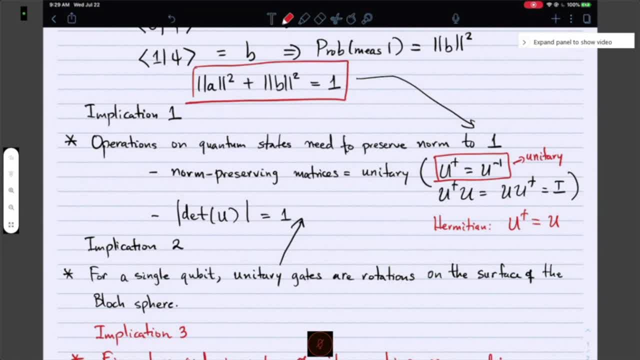 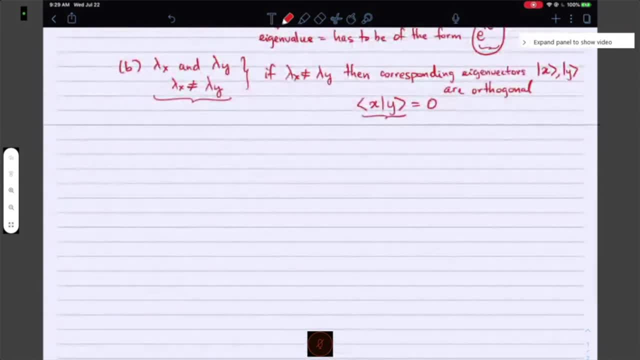 All right. So I hope that has been a good sort of review of the kinds of details that you've seen in your in your first lecture. Let's quickly talk about what you learned in your second lecture. So in your second lecture you went from discussing these kinds of details about eigenvalues and eigenvectors to kind of a bigger picture perspective. 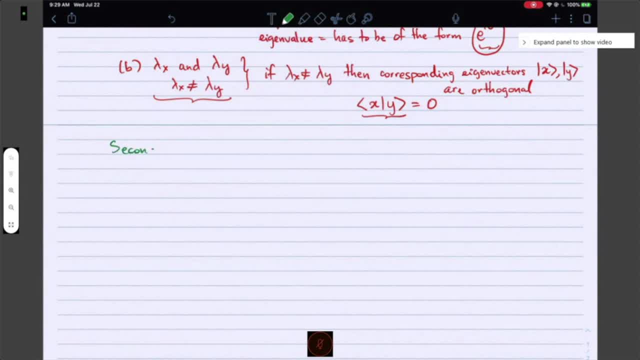 And you talked about the Deutch-Josa algorithm. You brought out a lexicon in Newton. So why is that the task? So what was the purpose of the Algorithm? What you were doing is trying to figure out if a function is either constant or balanced. 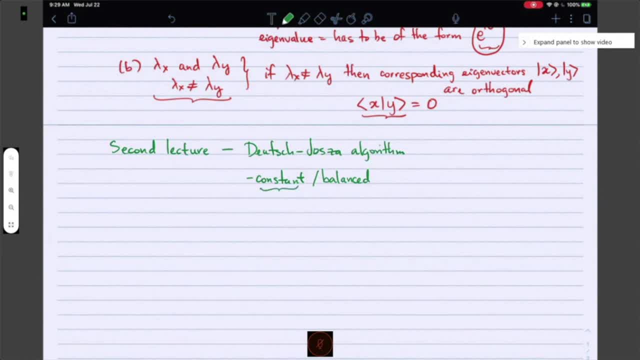 So what does that mean? It either also gave you the same output, so that's constant, or it was balanced, meaning that it gave you one output half the time and another output half the time for half of your inputs. And the really cool thing that you learned is that you can use a quantum computer to 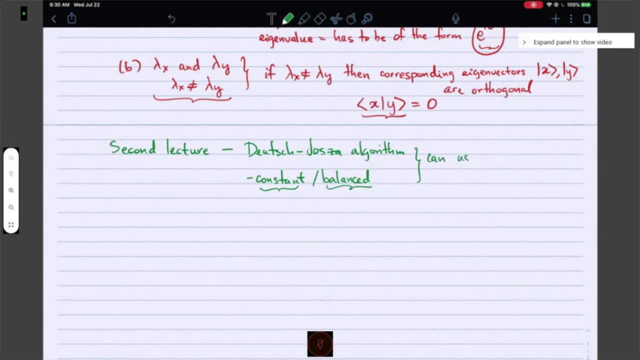 determine if can use a quantum computer to determine if a function is constant or balanced in one shot, And that's a really cool thing to learn. This is one of these things that really got the field excited and people really started kind of paying attention to the fact that quantum algorithms may very well be powerful. 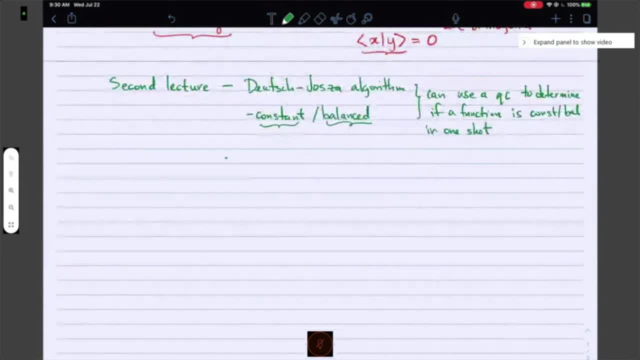 You also learned about one of the crown jewels of the field, called Grover's algorithm, And in fact, this was the focus of your second lab. What was the point of Grover's algorithm? The point of Grover's algorithm? The point of Grover's algorithm, was to tell you about how to do unstructured search. 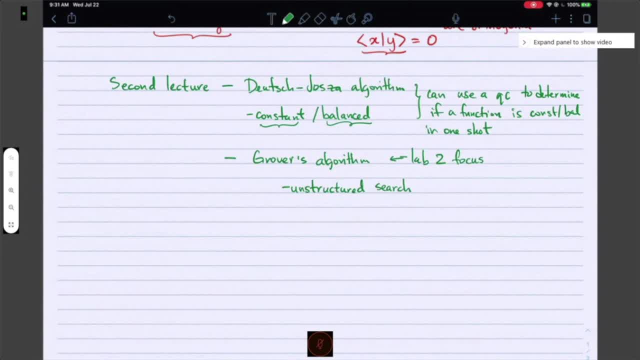 What does unstructured search mean? It means you're given a list, for example, something that looks like this: 14958.. There's no pattern that you can take advantage of here. There's just no structure. That's why people call it unstructured search. 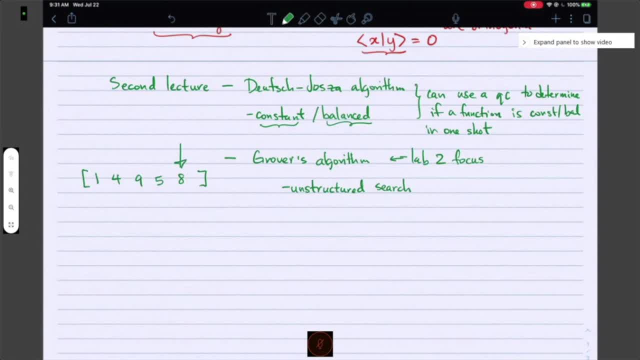 So to find a number maybe that you want to look through in this list, you really have to say, is it this number, Is it this number? No, Is it this number? No. And you really have to look through the whole list until you eventually stumble upon the. 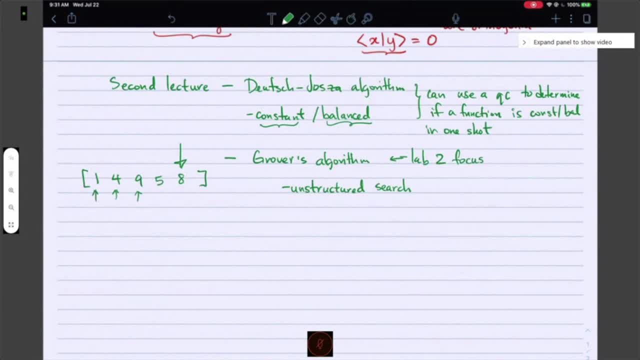 number that you're interested in. So classically, in the worst case, you'd need to look through all of the numbers in that list at least. So you need to at least look N number of times if you have N items in that list. 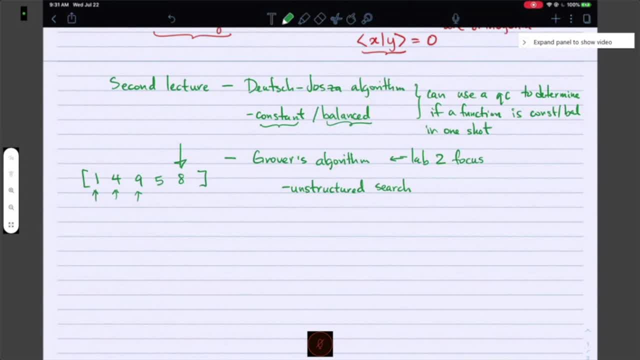 Using a quantum computer and Grover's algorithm, we know that we can do unstructured search in N items With Okay. Okay, isn't that right? That's nice. Yeah, it's a great question. So in the worst case we use the example I gave in the in the first class of O of square. 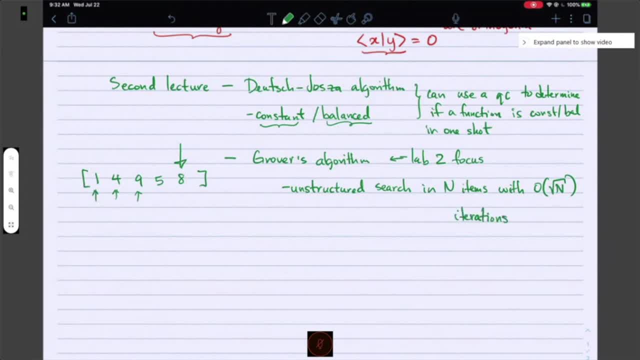 root of N, which just means in the worst case, the dependence of the number of iterations that you need is square root and not linear in it, And that's a really profound thing. That's really awesome to learn, All right, So I hope that kinda reminds you of what you've learned so far in your first two lectures. 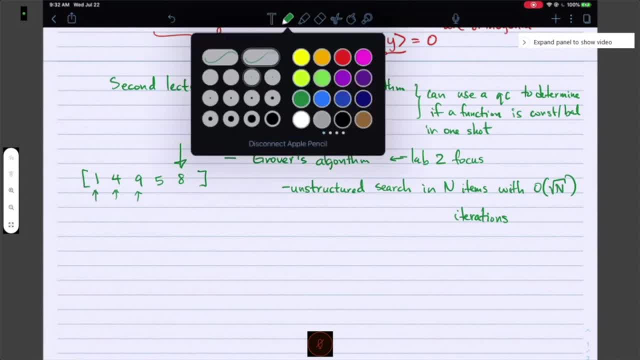 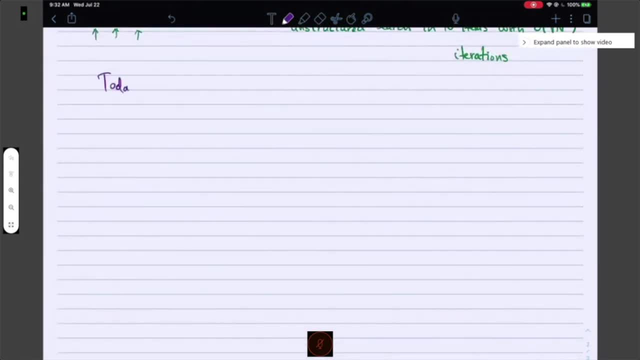 the preliminaries for Shor's algorithm, which is what we'll be covering in today's lecture. So let me change the color here and say today we're going to be focusing on preliminaries for Shor's algorithm. I'm sure many of you have heard about this algorithm. 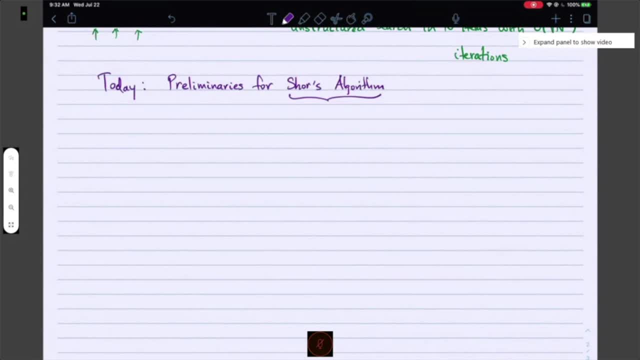 and we'll go through the algorithm in quite a bit of detail and I'll show you some examples to help clarify the concept. I'll just point out here that this is a famous algorithm and really one of the algorithms that brought into perspective just how powerful quantum computers can be in the 90s. 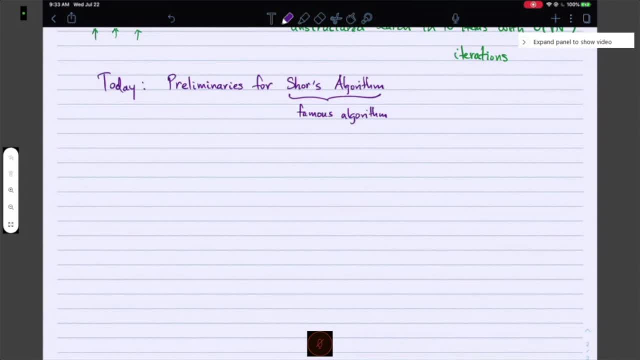 Okay, before I continue down this path of talking about Shor's algorithm, Brian, can we take a couple of questions here just to clarify some concepts for people? Sure thing, absolutely. I think one question that might be helpful at the beginning here: 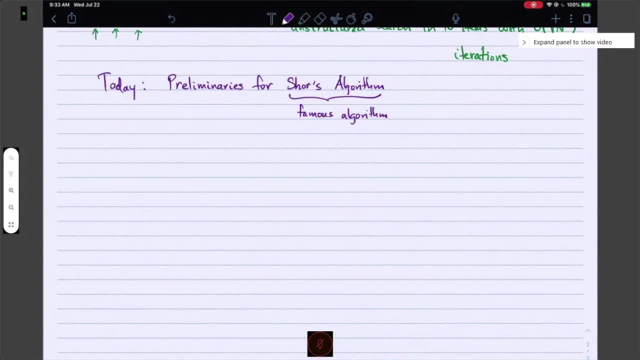 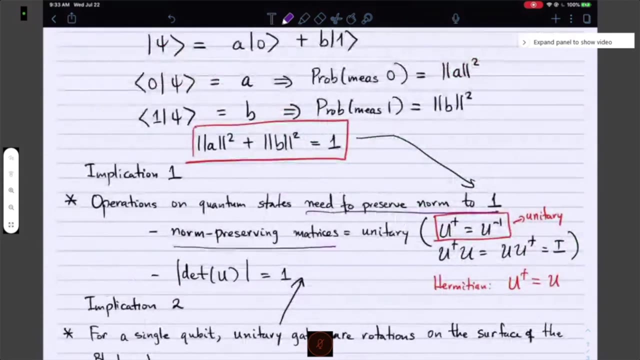 are unitary matrices the only norm-preserving matrices. Yes, so unitary matrices, by definition, are norm-preserving. That's why, when we immediately said on quantum states, we need to preserve the norm and therefore our matrices have to be norm-preserving. 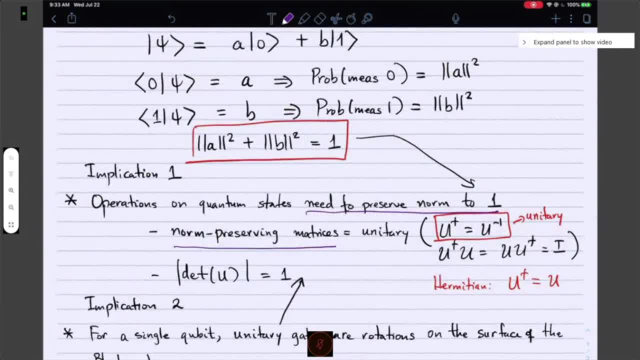 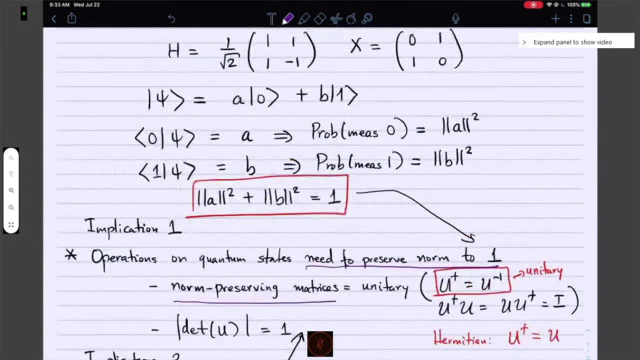 that's definitely nailing down unitary matrices. It's pointing you in that direction. Great. So then one more question that we had. I think that just for you to be aware of to answer. maybe at the break someone was asking about all the books you have behind you. 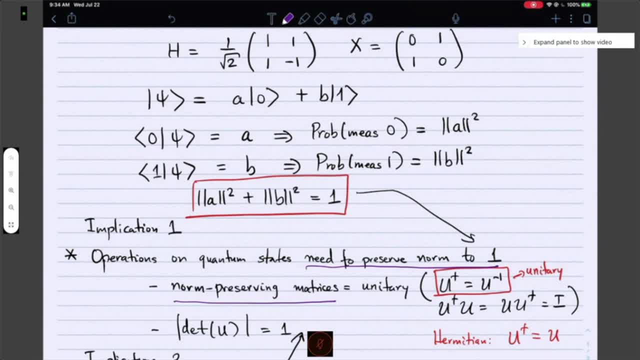 I want to know the books you use to help get you to this level. So don't answer that one now, but maybe when we get to our first break you can have that list ready. Sounds good. There are a lot of them, and a lot of them are useful for different contexts. 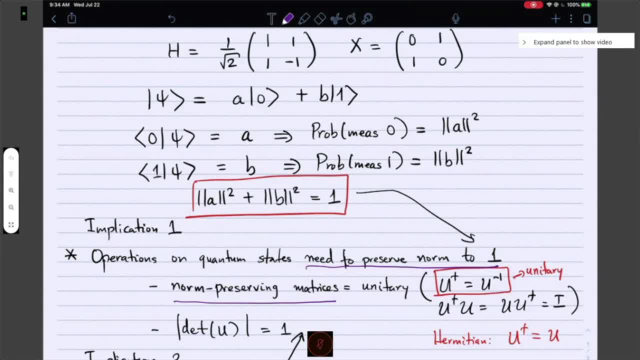 I can talk about why each one is useful, at least for me, over the break. I can talk about why each one is useful, at least for me, over the break. I can talk about why each one is useful, at least for me, over the break. 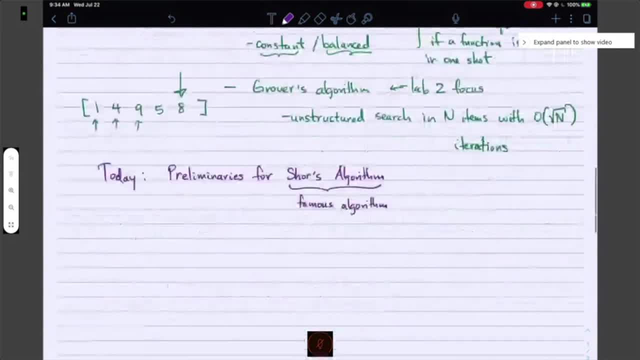 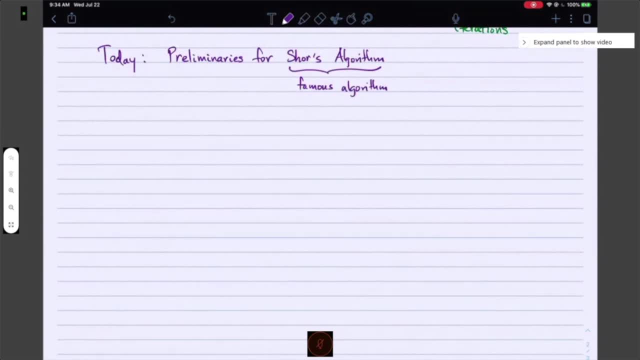 Okay, work. Okay, let's go back to the lecture material. All right, so Shor's algorithm. why do we care about Shor's algorithm? What are we trying to do? Well, Shor's algorithm can serve in many different. 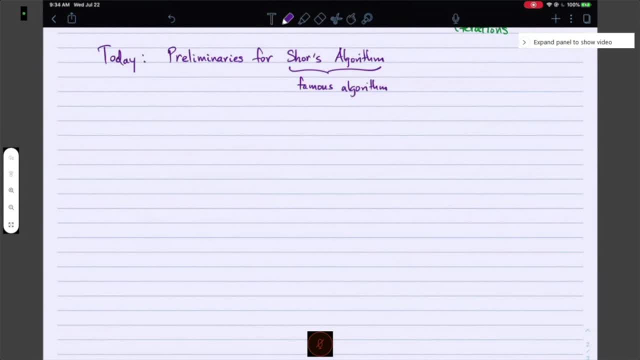 quantum programs in different ways, but the most popular one, perhaps, is to solve the following kind of problem. So let's describe what problem we're trying to solve. If I give you a function that is periodic, I would like you to give me its period. So find its period. 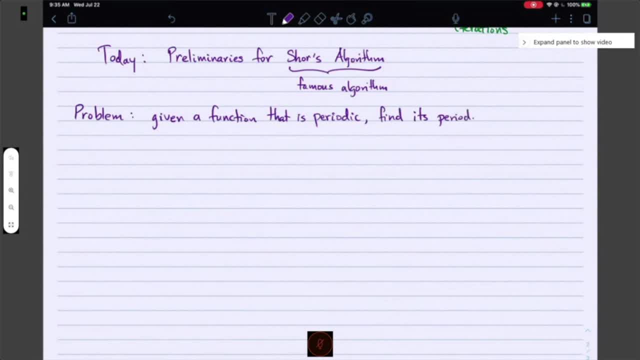 This is a deceivingly short problem That sounds like it has a solution that should be very easy, but it's actually a very challenging problem. So let me give you kind of a stricter definition of this problem. Let's be a bit more specific. So let's say that I have a solution that is 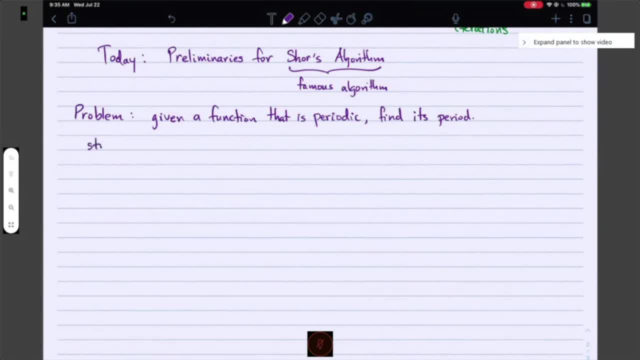 more concrete. So I'll say: strict definition. We will call that function f and it takes an argument x, And I will say: if f of x is equal to f of y, for x is not equal to y if, and only if, x. 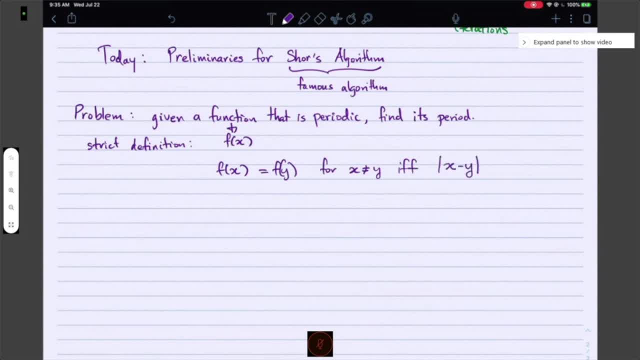 minus y, And I am going to say that y is equal to x minus y. The difference between them in absolute value- because I only care about the difference- is p times some constant. So p here is the period. So this kind of precise definition is actually a very, very complicated way of saying something. 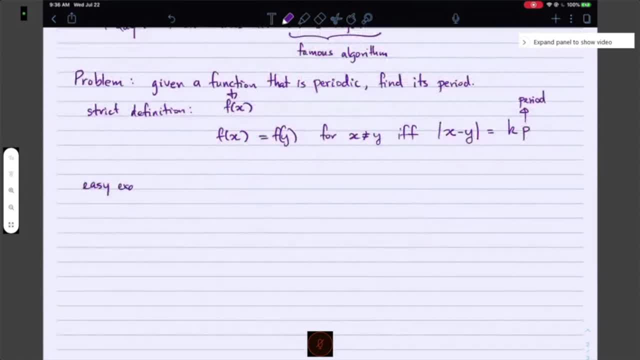 very simple that I can show you visually. So let's do an easy example function. I'll just draw it out for you And let's say the function is a function of theta and it's actually a function that you know very well. 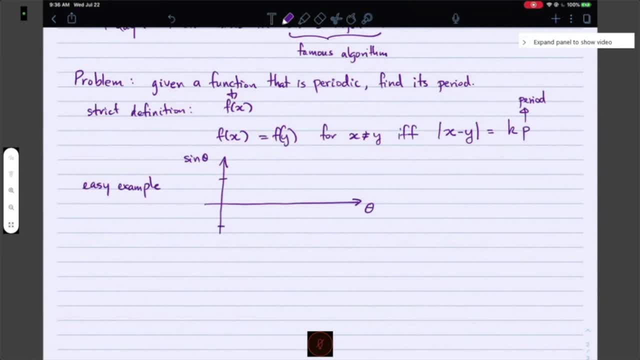 called sine of theta. What does sine of theta do? Well, it ranges from minus one to one and it looks like this: Okay, so this is one of the easier periodic functions to deal with, right? So the period is immediately notable. 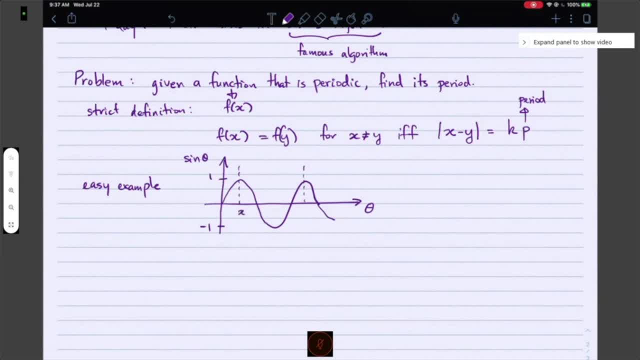 If there are two values here, let's call them x and y. The period here between x and y for a function sine theta is two pi. So I can always tell you, maybe if this function keeps going later and comes back down and maybe there's another y here, 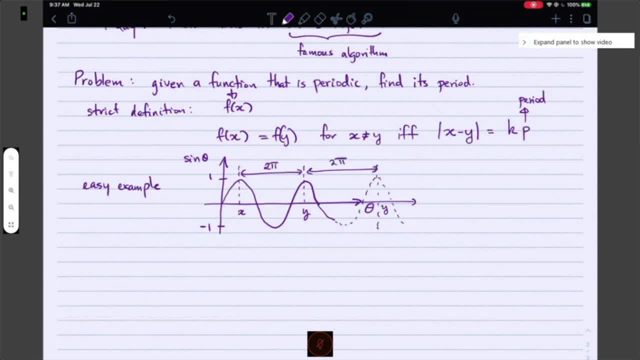 there's another two pi here. So all that means is the difference between x and y in this case is two pi times some constant, where that constant is some integer that we're not going to focus on too much. We said x and y and the absolute value. 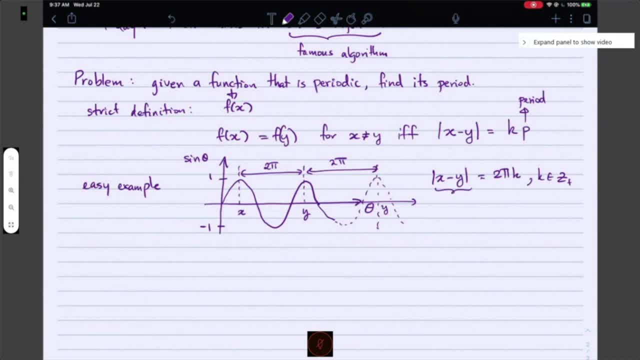 so this has to be a positive number, obviously z plus and zero. But at the end of the day, the concept that I'm trying to show you here is that the periodicity here is very clear. You can all very clearly see the period. 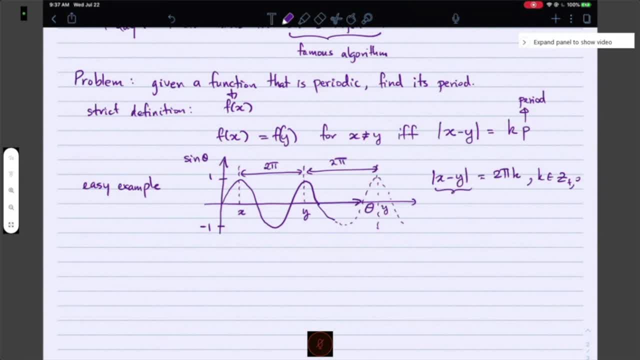 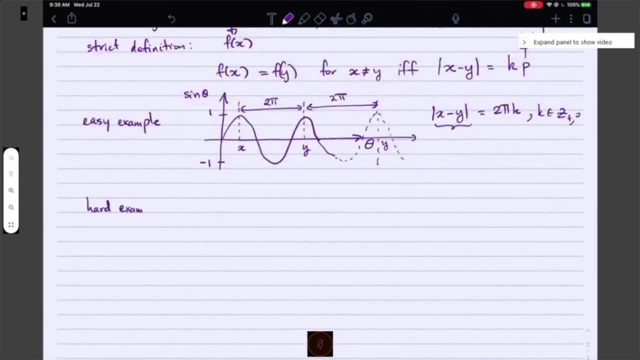 and tell me exactly what the period is. But let me show you a bit of a harder example. So let's do the following, Let's say hard example. It's going to be a bit tough to draw this, So let's hope that I can do this well. 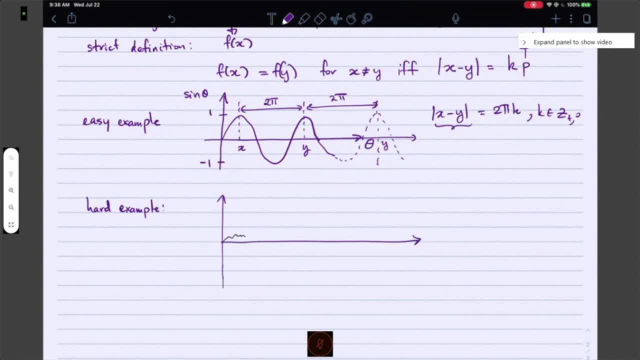 Let's think of a function that does something that looks like this And then starts over again and does exactly what it did over on the left side. So if I gave you this function with your eyes, you could look at it and tell me: this is the period. 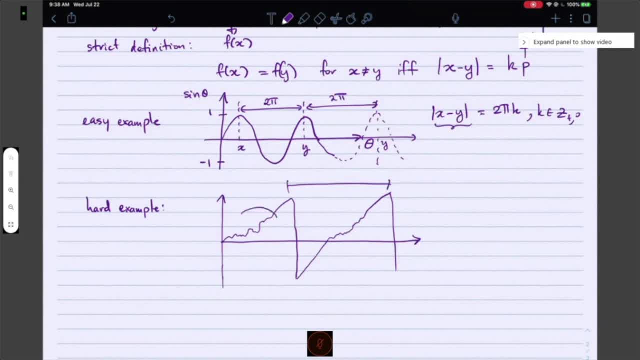 But in fact, if you were zoomed in and you were looking only in this small region, for example, what you would see is something that looks like this If you were to draw the�: Well, if you see that zoomed in region, 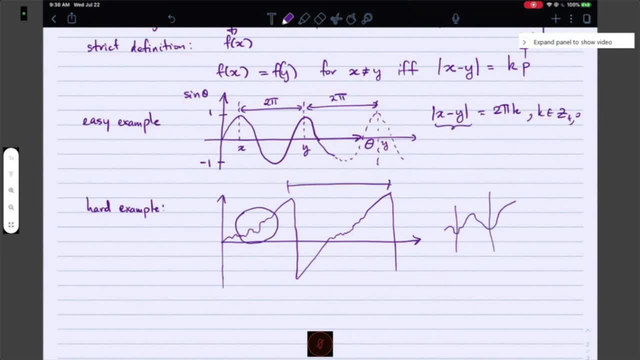 does that mean this is the period? So you can see here that functions that are not necessarily sinusoidal can be quite confusing in order to tell the period. So there's a bit of a difference here between the easy kinds of problems, the sinusoidal problems. 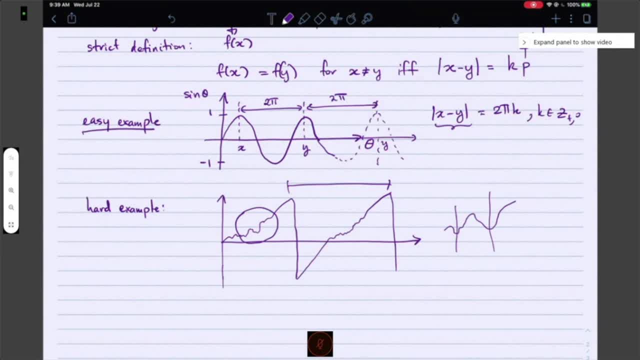 And for those of you who deal with audio processing, signal analysis, some of you have already seen that you can take advantage of how easy to see- because it would make sense- is to work with these kinds of functions and to find out what their periodicity is and to 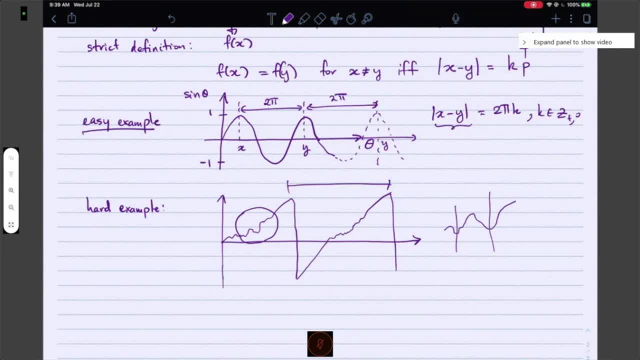 take advantage of them as decomposing other complex functions. This hard example should show you one concept, which is that you might be trapped in local regions when you're trying to determine the periodicity, so you really need a lot of data points in order to tell the period. 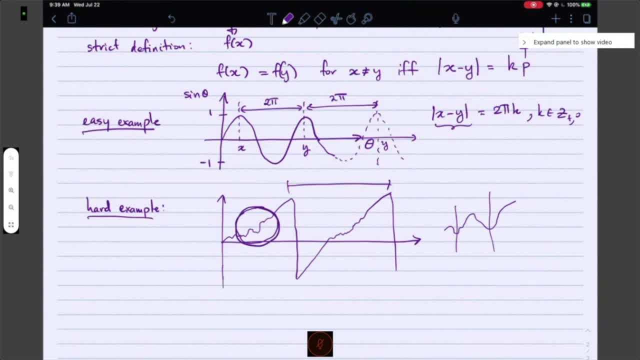 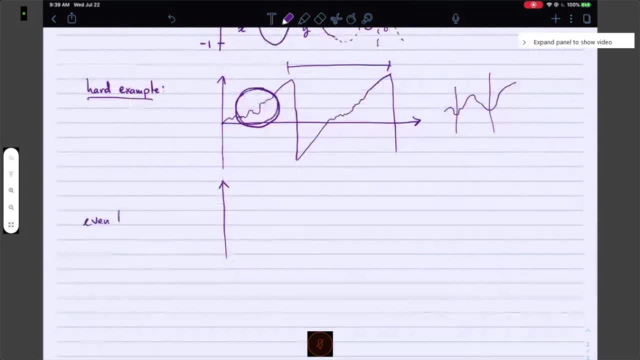 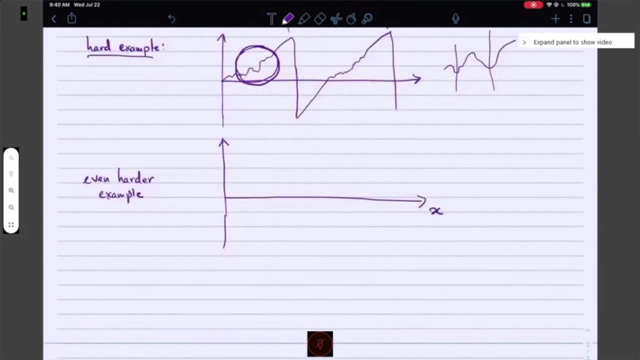 of something that's more complicated like this, And sometimes there are examples that look like this. Let's call this an even harder example And I will be very careful to draw my axes here: X and F of X. here, Let's say, the function looks like this: What's the period here? Is there a period here? 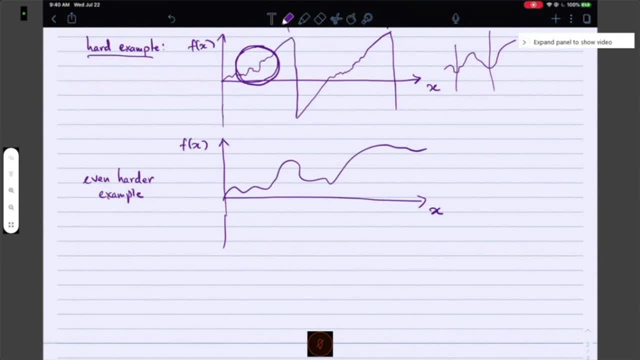 Well, first of all, when you look at this function, it's very hard to see anything periodic by eye. But in fact, what you don't know is that you may very well be too zoomed into this function. So, in fact, if you went out further, you might have noticed that it would actually start repeating. 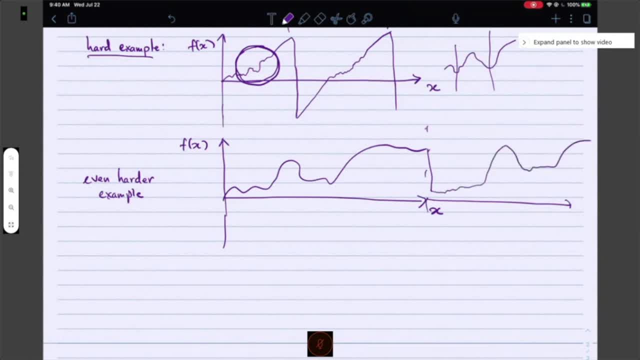 and do exactly what it did before. So now the period looks something like this, And what you can see here is that the period is very, very small, And so you can see that the period is very, very small, And so you can see that the period is very small. 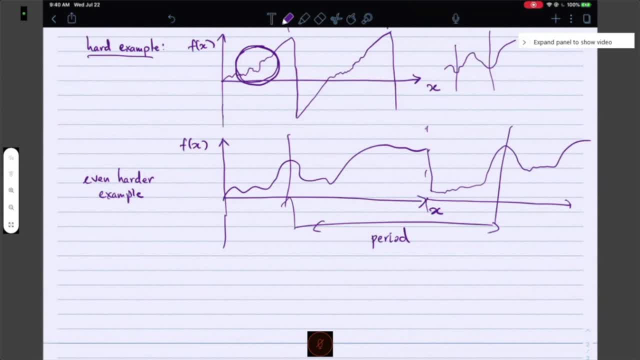 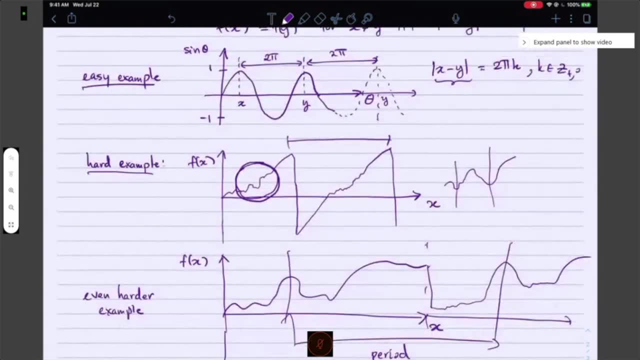 In fact, we can see that the period is very, very, very small. So let's just say that if you look at this function, it's very, very, very small. So I hope all of these examples show you exactly how the problem of finding periods can be very. 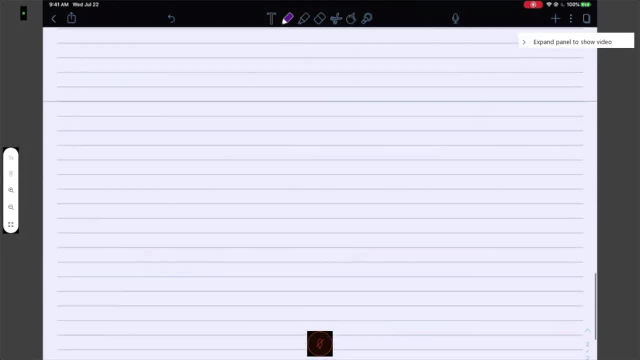 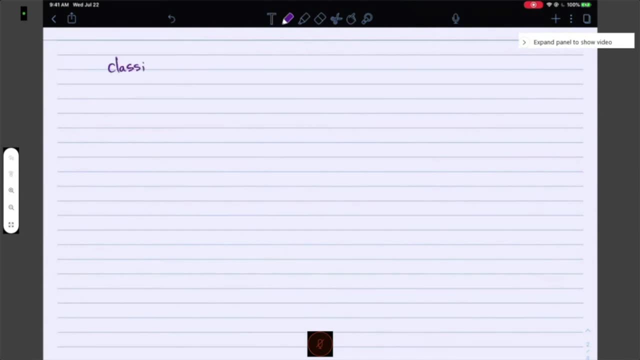 complicated, when these kinds of things are not necessarily as easy as dealing with sines and cosines, like we saw in that very first easy example. Well, if you have to classically find out what the period is, it's going to take you. 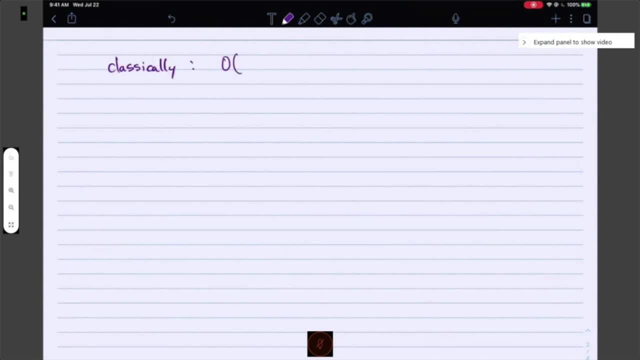 something that looks like. so remember this is the same worst case notation that I used before. It's of an exponential that looks like C, some constant times N to the one-third and log N to the two-thirds- A very complicated way of saying there's an exponential here. 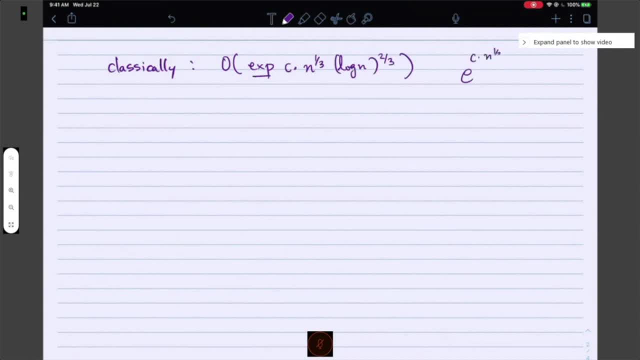 So it's E to the C, N to the one-third, and then there's a log of N to the power of two-thirds. So you can see there's an exponential dependence in how hard this problem becomes, as you need N bits needed to describe P, the period. 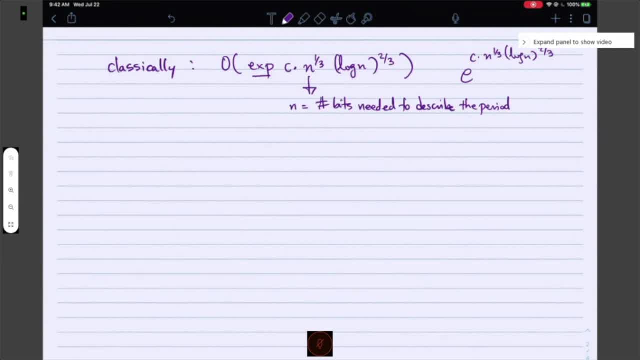 So this is. some of you might be familiar with things like Fourier transforms and dealing with fast Fourier transforms. These are the techniques that can get you this kind of benefit. So this is how you do things classically In the quantum example. This is where Shor's algorithm comes in. 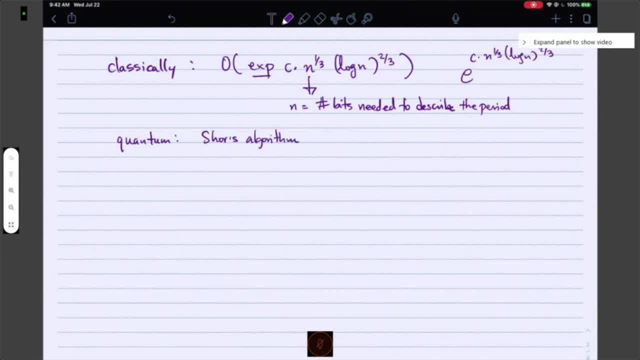 Right Right Shor's algorithm can do this in O of N square log, N times log log N. And when you see something like this, it's important not to be distracted by these factors log. What I want to point out to you is that 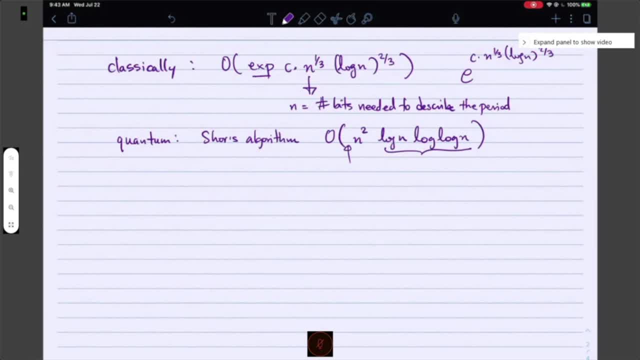 there's no exponential here. It's now something that's faster than O of N cube. It's a little faster, It turns out. these coefficients can be quite large sometimes. So let's say this is a little faster than O of N cube. 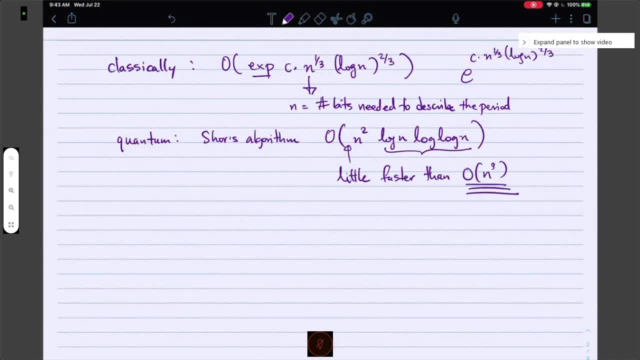 Well, this is already exciting, right? So here you had an exponential in N. It's a cube root of N, but let's just say it's an exponential. Here you don't have that exponential dependence anymore. You've turned that into a polynomial problem. 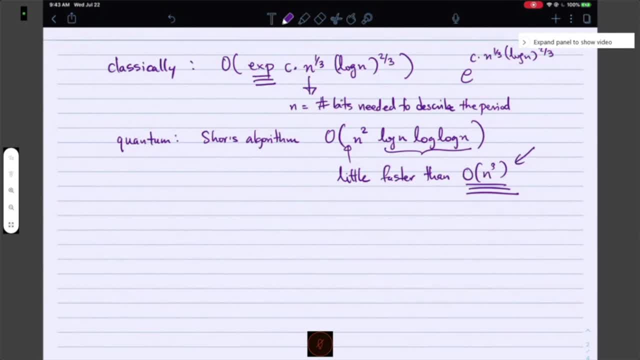 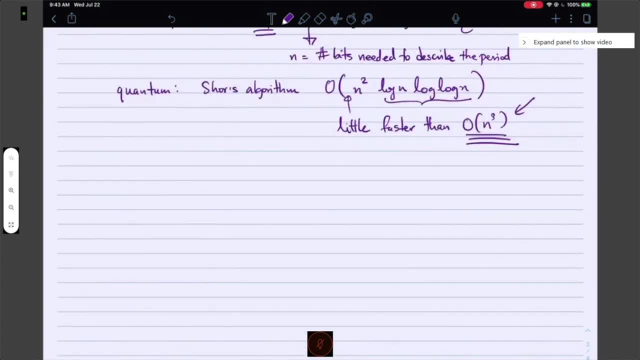 So this is the kind of thing that people call polynomial exponential speedup. So this is an almost exponential speedup, and what you have is this benefit, where Shor's algorithm speeds up this particular problem of finding periods, And the reason why this works. 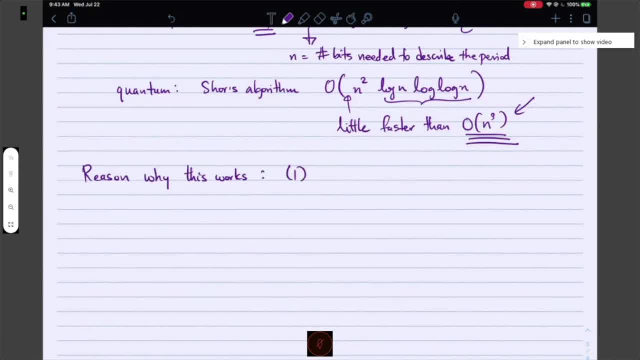 there are two reasons why this works. The first reason is quantum Fourier transform, which is at the heart of Shor's algorithm, And the second reason is another piece that we'll learn tomorrow, called modular x-minitiation. So I just want to point out one thing to you. 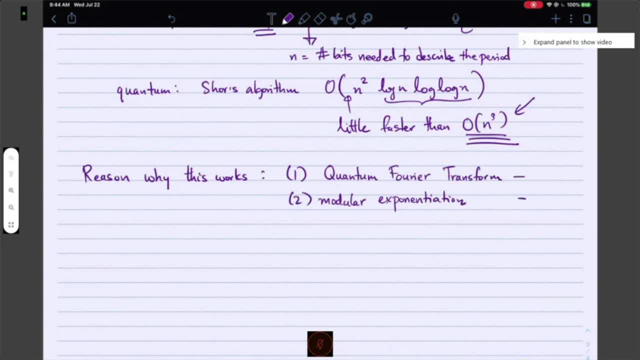 These blocks of Shor's algorithm are quite involved. Today we'll cover this one and tomorrow we'll cover modular exponentiation. So we'll go through these blocks, So we will do that. So these reasons are why Shor's algorithm works as well as it does. 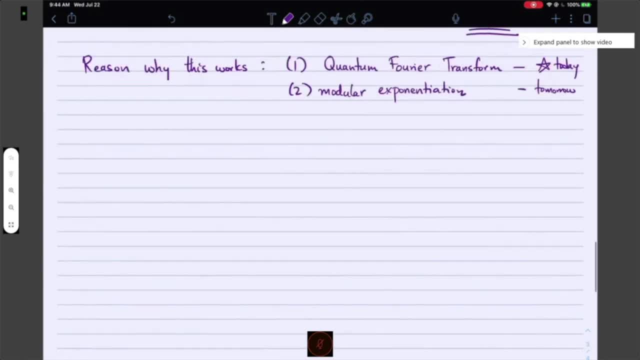 And what is the implication of all of this? Well, first of all, I want to point out to you that the problem of factoring a number which is a product of two prime numbers, this problem is the basis for the security on our computers in several places. 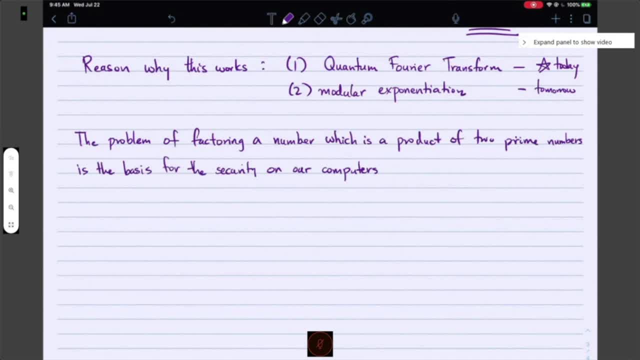 So what does this mean? I just, you might've noticed, I just switched a problem on you. I was talking about periodicity up here and now I'm talking about factoring numbers. It turns out- tomorrow you'll learn- that the idea of periodicity and the idea of factoring numbers 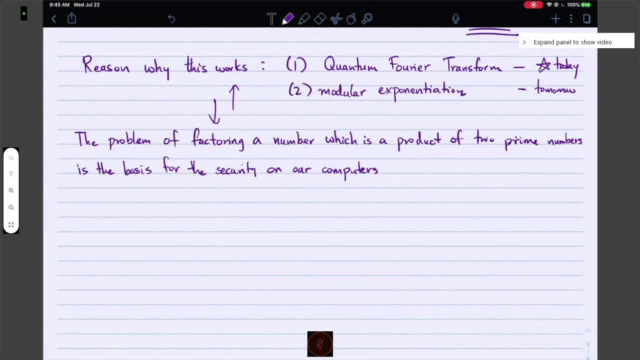 are very much related And in fact, the idea of converting between one and the other is why Shor's algorithm is so successful. But given that this problem of factoring is why? is the basis of the security on our computers the fact that you can now solve this problem? 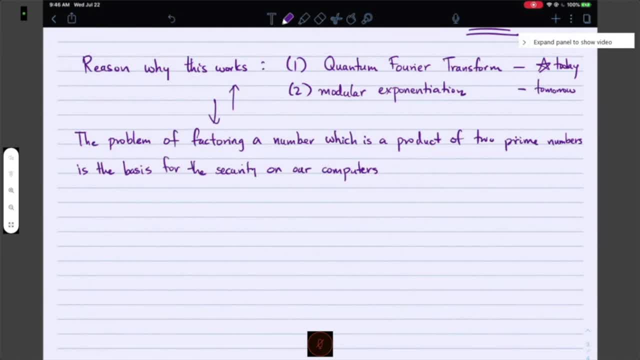 much more easier, in a much more easier way on a quantum computer. this is one of the reasons why there's a strong implication for knowing and getting quantum computers to work. So this is has serious implications for security, but is also not easily accessible today. 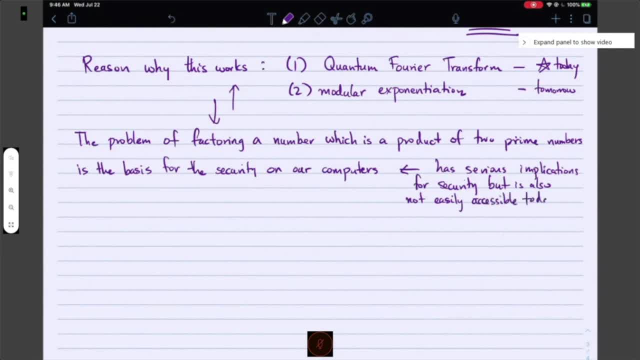 And the reason it's not accessible today- as you'll learn in the next- this lecture and the next day's lecture- is that it requires several qubits, and several good qubits. Okay, so I hope this clarifies why we're here. 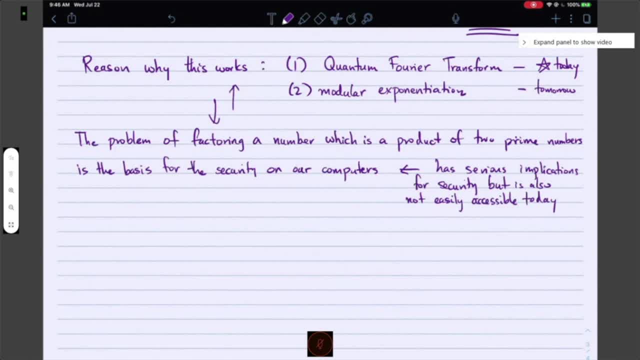 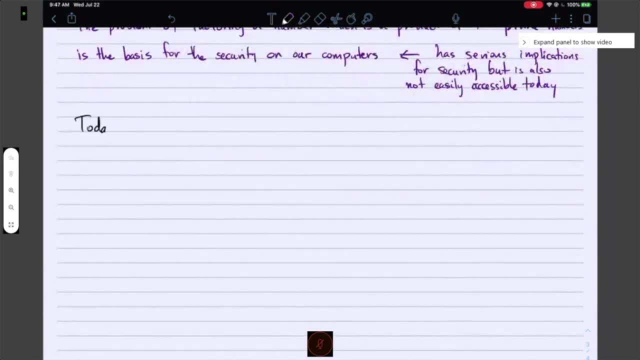 the reason why we're doing today's lecture. So again, as a quick reminder, let me write down in a different color: Today we're going to be talking about the quantum Fourier transform And quantum phase estimation. Now, I haven't talked so far about quantum phase estimation. 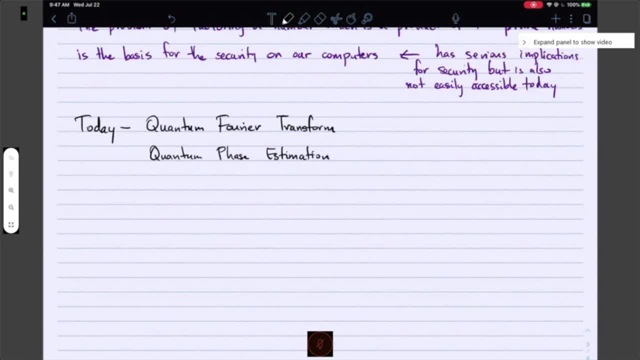 in the story that I told you, but you'll find that quantum phase estimation is actually what Shor's algorithm is in disguise. So I really want to make sure that you see Shor's algorithm Okay, but I'll make sure that you have a very good understanding. 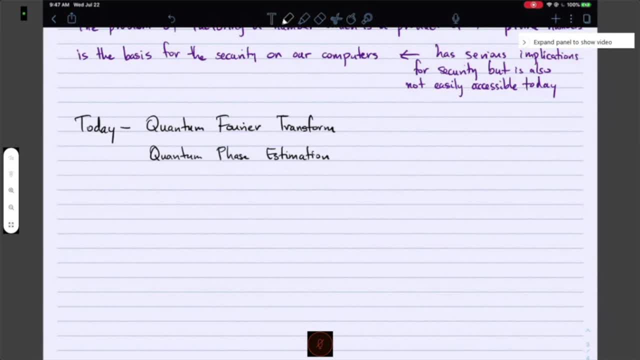 of quantum phase estimation today. So I'll just put a caveat here by saying Shor's algorithm is really just quantum phase estimation in disguise, And this will, I hope, become very apparent as you work through the lectures today and tomorrow. All right, let's take a quick pause here. 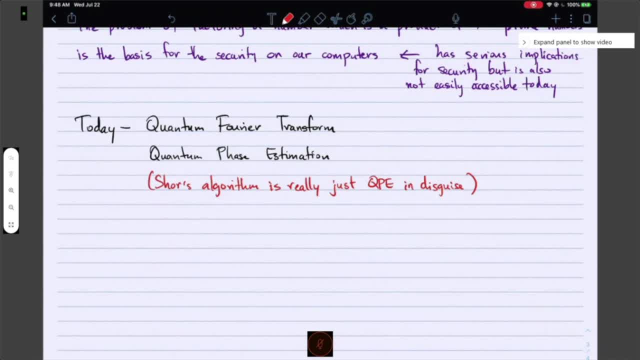 and see if any questions have come up. If not, I'll start talking about the quantum Fourier transform Brian. are there any outstanding questions? I'm going through. I'm looking for people asking questions about today's lecture here. So we have one question that's highly upvoted. 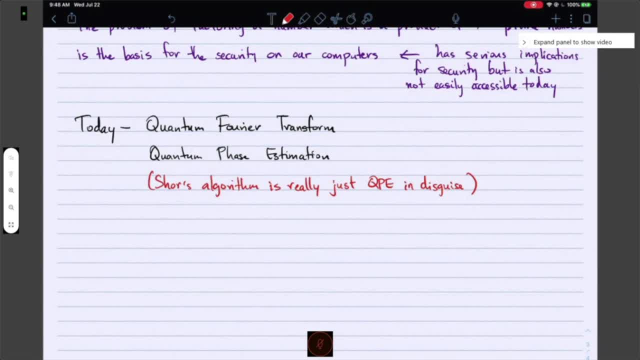 It's a long one, though, So if you open up the ask a question, you'll be able to see it too. Well, implementation of quantum Fourier transform in Shor's algorithm. why can't we use classical superposition? And they give an example of what they're talking about. 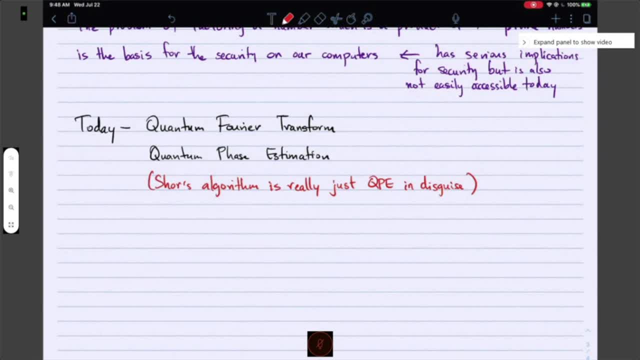 Using electrical pulses with phase difference will have the same or identical constructive or destructive interference patterns? I will. it's good to pause this question, although I would strongly recommend Brian maybe take a screenshot of this question so that we can answer it tomorrow, Because as soon as I'm talking about Shor's algorithm tomorrow, 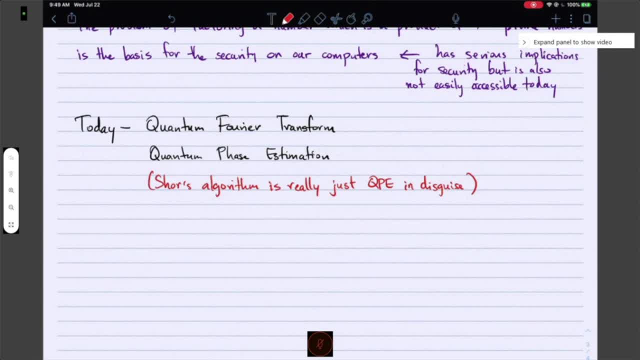 and putting boxes together. there's a point where I'll point out and tell people: this is where you couldn't have done this with a classical system. But for today it doesn't make sense to focus on this question. Great screenshot taken. 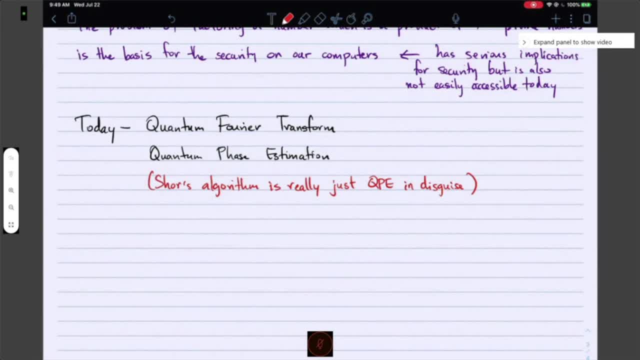 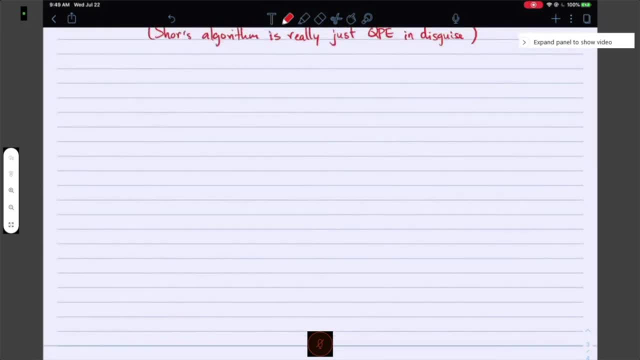 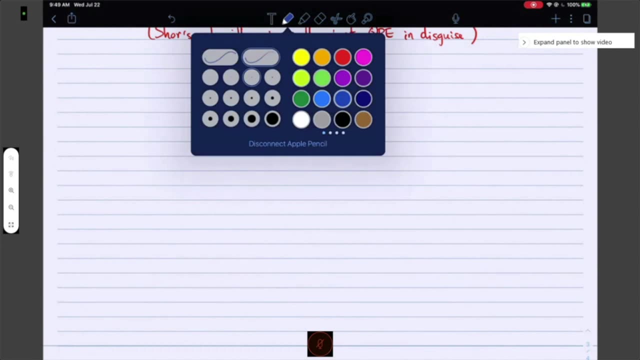 Thank you, Brian. If there are no other questions, I think we can continue. Sure thing, Okay. so what is quantum Fourier transform? Let me just very quickly I'll give you a few examples. Let me just very quickly start changing the color here. 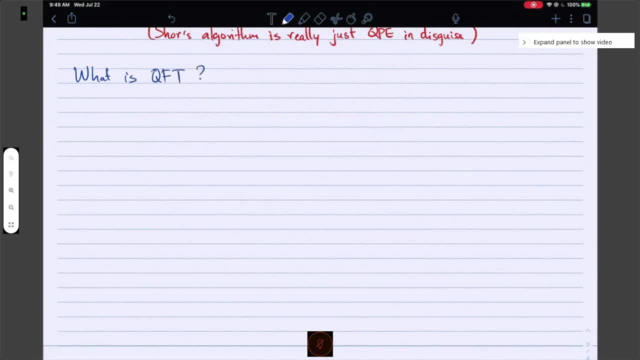 All right. so, like many things, I could give you a very complicated definition of what the quantum Fourier transform is here, But at the end of the day, the quantum Fourier transform is actually a very simple concept. A quantum Fourier transform is effectively a change of basis. 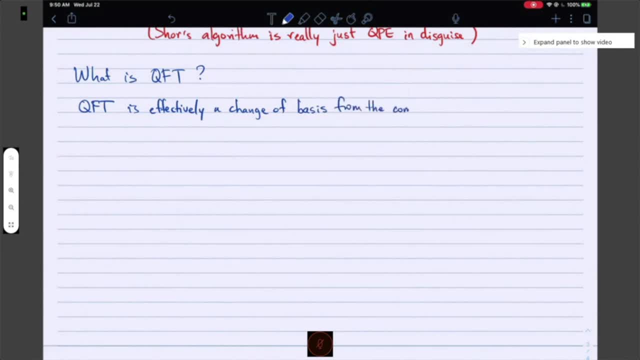 from the computational basis to the Fourier basis. Okay, that's a very short and succinct way of saying a quantum Fourier transform is effectively a change of basis. Done, end of story. What does all of this mean? What does the change of basis mean? 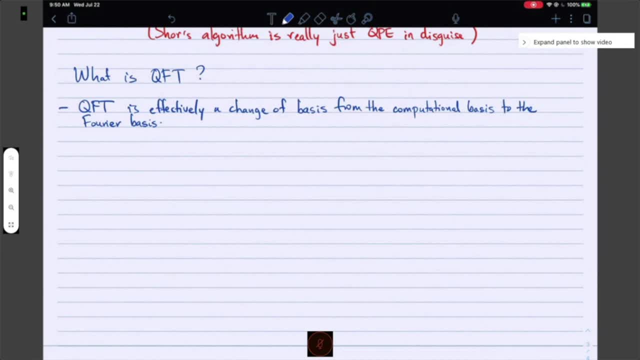 What is computational and Fourier basis? Let's go through that in a bit of detail. But one thing I want to make sure at the end of this lecture is that all of you can repeat: quantum Fourier transform is effectively a change of basis from computational to Fourier basis. 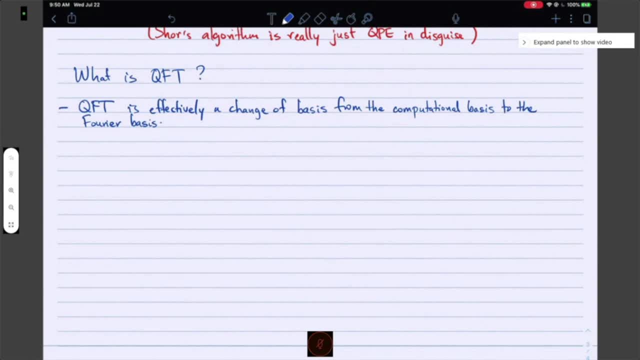 It's really that simple. All right, let's talk about the computational basis. You've already seen this. What is the computational basis? Let's talk about one qubit. Let's do an example of a one qubit Computational basis states. 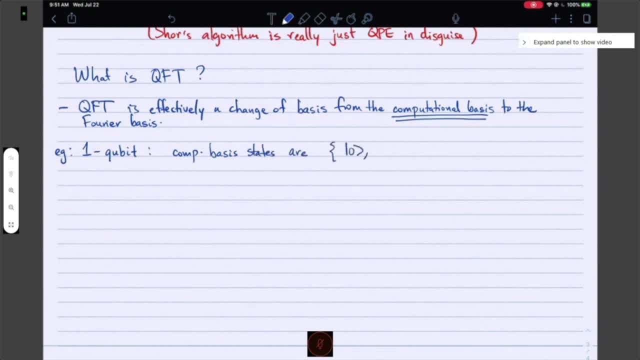 are zero and one. That's it. It's really not that complicated. Zero and one are the computational basis states. Fourier basis is something you've also seen. You may just not have. well, I'll just call that one anyway. You may not have a spot there. 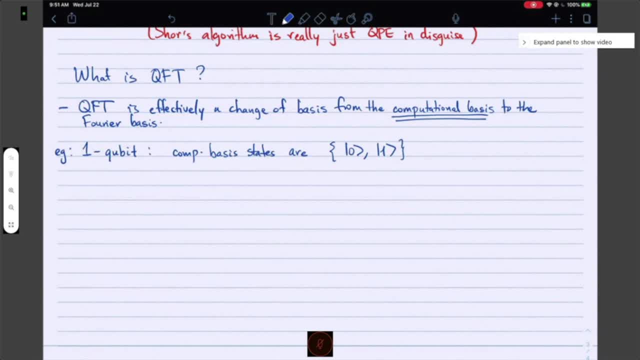 you just haven't been told that this is the Fourier basis. The Fourier basis is actually the plus and the minus states. It's really that simple. I'm just telling you a fact here. but let me show you the connection between the two. 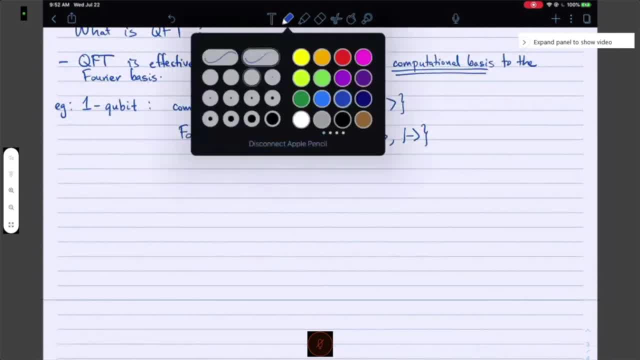 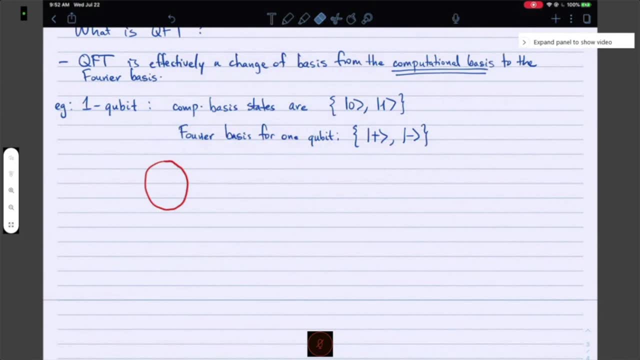 So I'd like to start by drawing zero and one on the Bloch sphere. So here's a Bloch sphere, or at least my impression of a Bloch sphere. It's a pretty bad drawing as it is now. Let's say this is zero and let's say this is one. 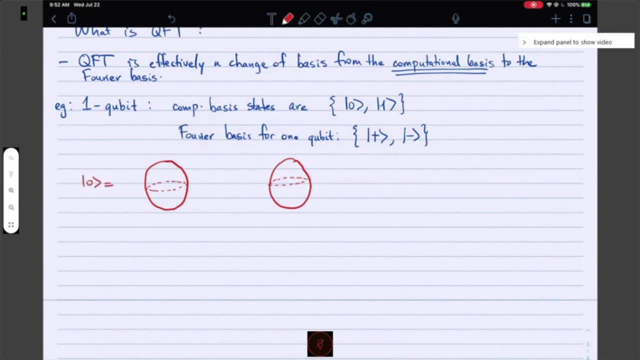 So zero looks like this and one looks like this. So where is zero? Zero is pointing to the top. Where is one? One is pointing to the bottom. So you've seen the Bloch sphere and how these states can be represented. What is the Fourier basis doing? 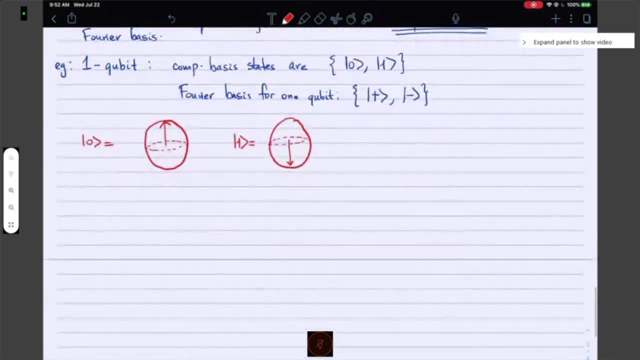 The Fourier basis is actually doing something very simple: Instead of taking you between the two poles up and down, it's taking you between the two sides on the equator. So you're either here or you're here the other way, pointing the other way. 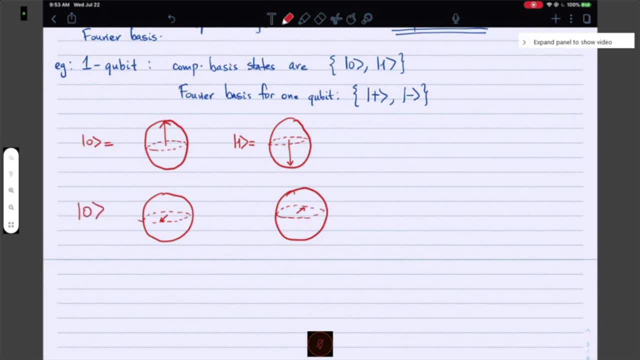 So I'll write a notation here. This will be the first time that you're seeing this. The Fourier basis version for zero: I'll call it zero with a tilde on top. The Fourier basis for one: I'll call it one with a tilde on top. 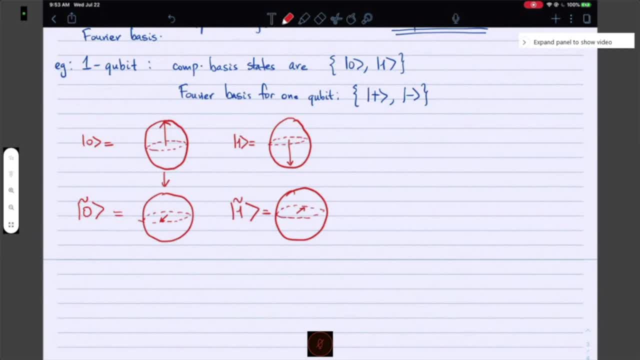 And that's what this looks like. So this is exactly what doing a query is doing, Okay, So this is the first time that you're seeing this. So you're going from this notation, where you're going between top and bottom, to being on the equator. 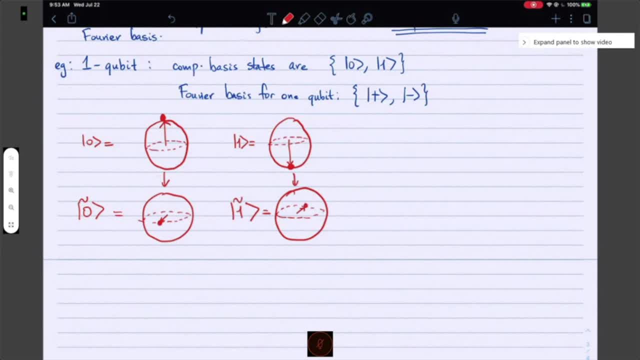 and having phases that go around the equator, And, in fact, some of you might have already noticed. well, wait a minute. I know how to make that transformation. I know how to go from the computational basis to the Fourier basis, at least in the picture that I've shown you here. 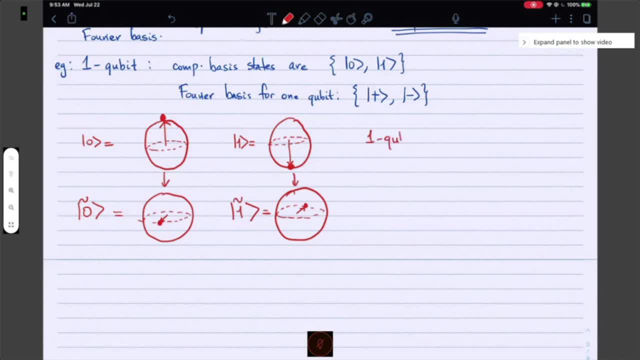 It's actually very simple. So a one qubit quantum Fourier transform. that does this. Any guesses? Can anyone put what guess you'd make for how to make this QFT transfer? So how would you go from the top side to the bottom side? 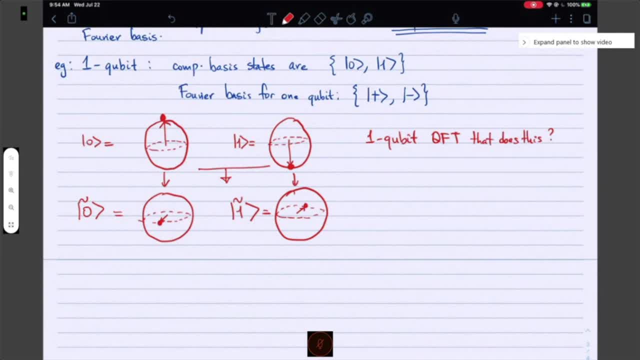 Bingo. So, Srishti, you have that exactly right. So, Hadamard gates is how you do a single qubit, QFT. So all of this is to tell you the amount of knowledge you've already gained by going through the material in the first two lectures. 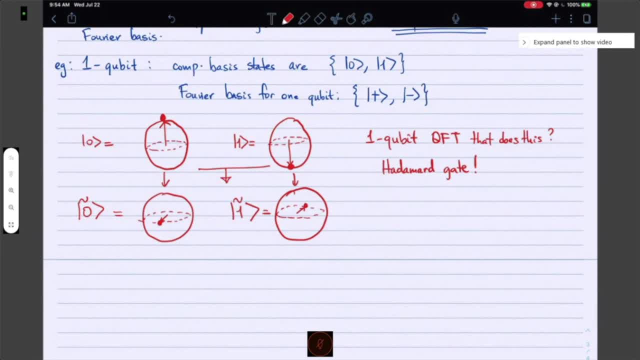 You may not have put it together, but this is exactly what it means to do a quantum Fourier transform, to transfer from one basis to another, And, in particular, the way you do that for a single qubit case is to do exactly what I've shown you in this picture. 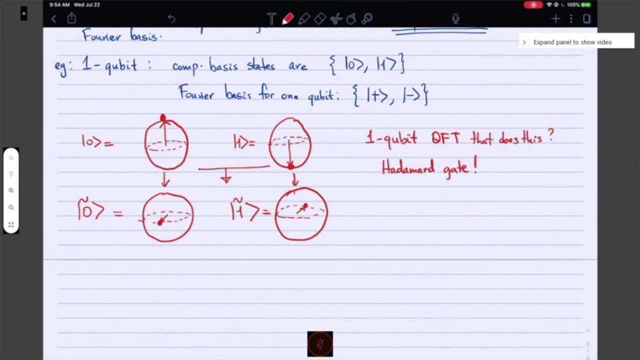 At this point, I think we're due for a break. So I think it's important to take a break, but before we do, I just want to put an image in your minds, So I'd like to start sharing my screen now. 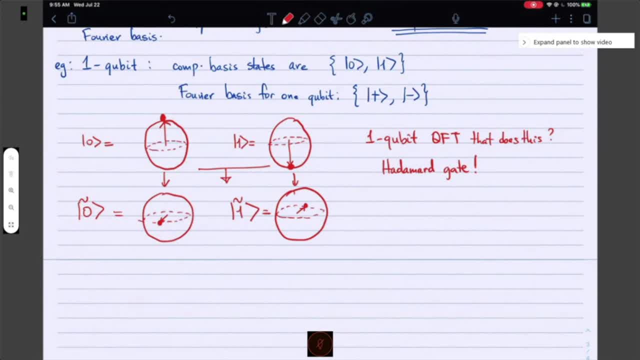 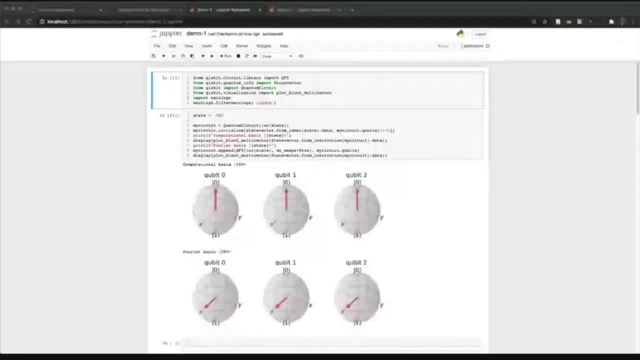 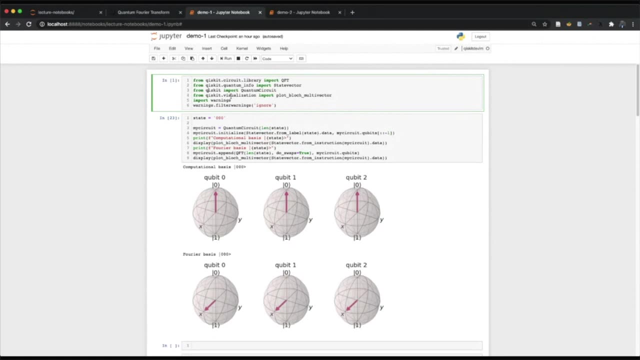 Brian, if you'd help me, I'm going to click the share screen option and I'm going to do this particular screen. So I've written a demo here to show you. So I showed you a single qubit QFT, but I'd like to show you what it looks like. 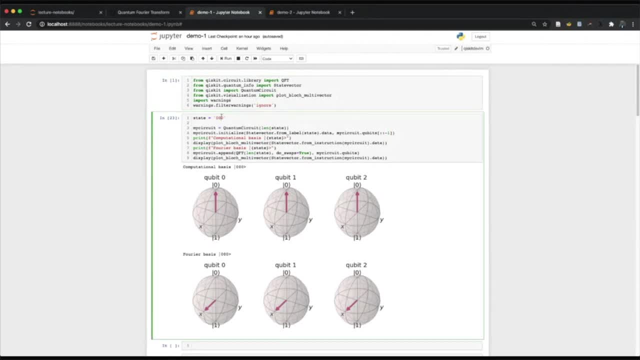 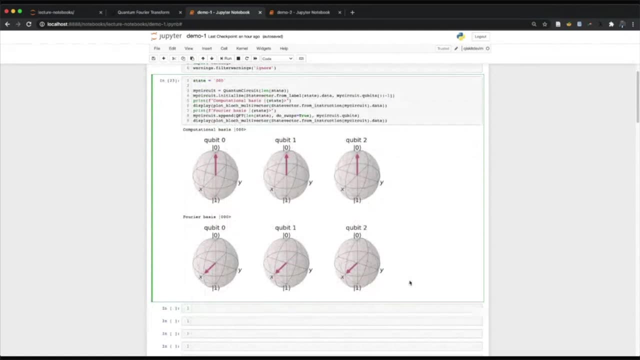 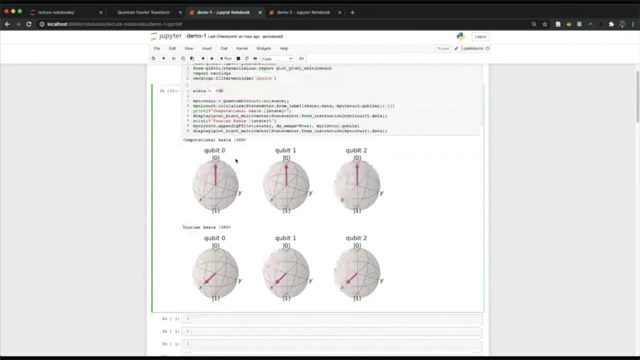 when you go to multiple qubits. So this is the state: zero, zero, zero in the computational basis, And this is what that same state looks like in the Fourier basis. You see, all the zeros went down to the equator. Now, if we instead look at a different state, 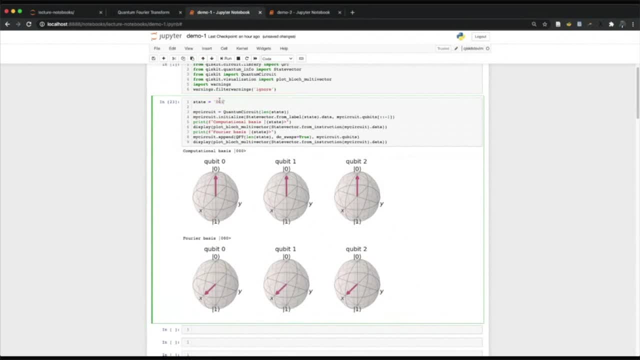 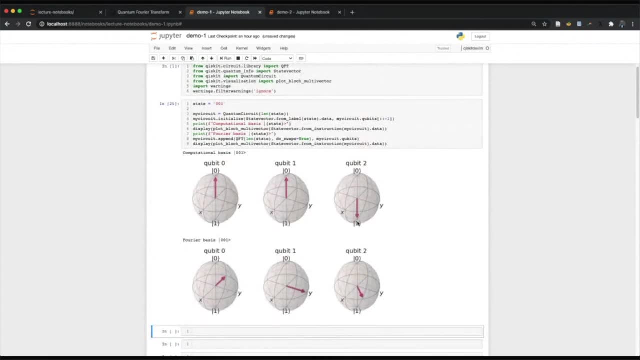 zero zero one. what would you expect? Think about what results you'd expect here. Zero zero one. So one of the qubits is flipped. So if you look at the Fourier basis, look at what happened. So this one was down here. 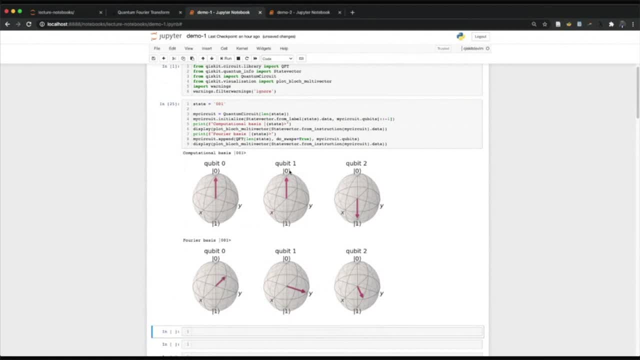 It rotated all the other to the other side. This one was down here. It rotated 90 degrees, This one did 180 degrees And this one, which started at the bottom and therefore started off on one side, is now getting a phase only of 45 degrees. 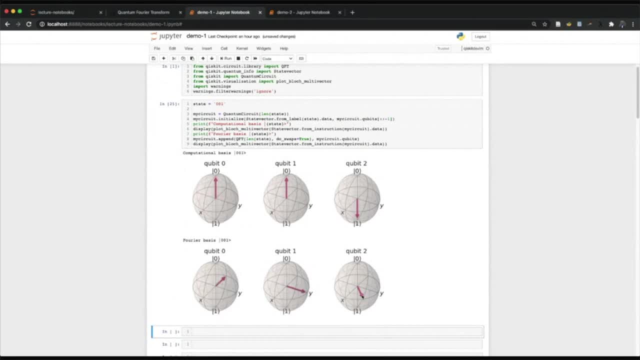 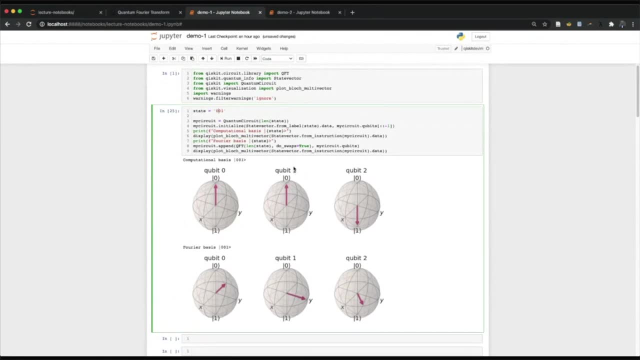 So 180 degrees, 90 degrees, 45 degrees. This is actually a very curious thing, So I could change this. So I could change this, I could change the state and keep showing you different examples, But I think the best way to demonstrate to you, 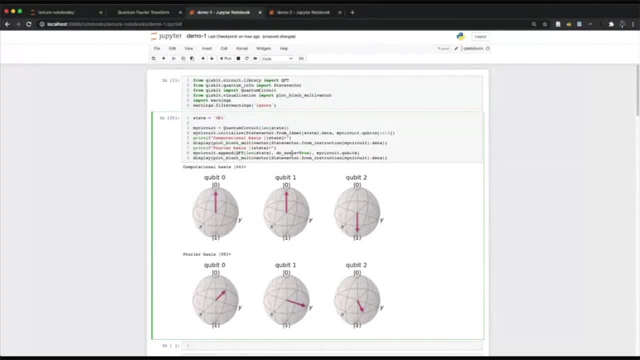 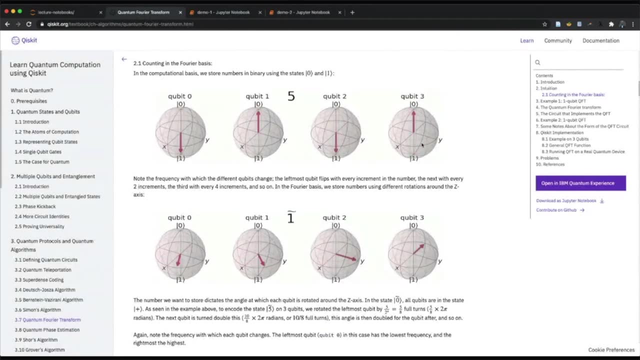 the difference between the computational basis and the Fourier basis is to show you a picture that we have in the Qiskit textbook. So this is a four qubit case where we're taking you all the way from zero up to two, to the power of four minus one. 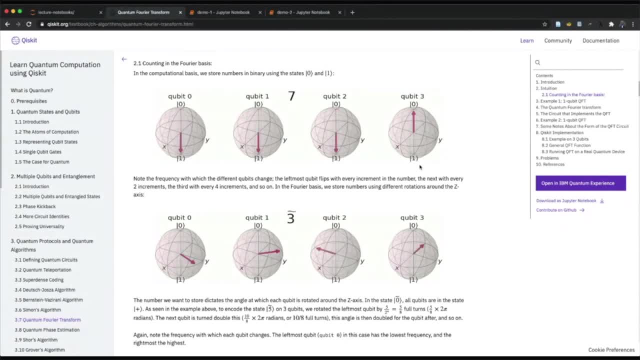 So up to 15.. You can see what from zero through 15 look like in the computational basis. All you're doing is flipping between zeros and ones, right? So you're basically doing binary counting In the Fourier basis. instead, what you're doing is rotating. 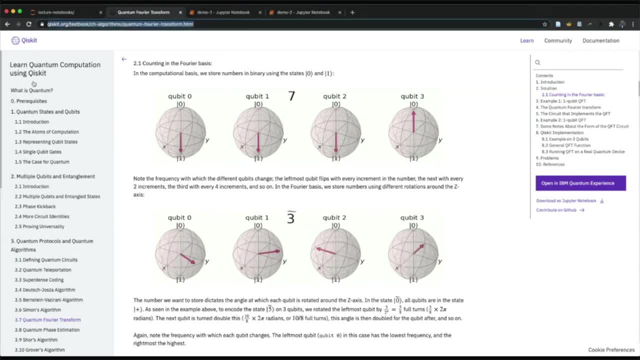 on the equatorial plane. I'm going to drop this link in the chat so that you can take a look at exactly this animation. But what's important here is for you to see how powerful it is to be able to do this. So in the computational basis. 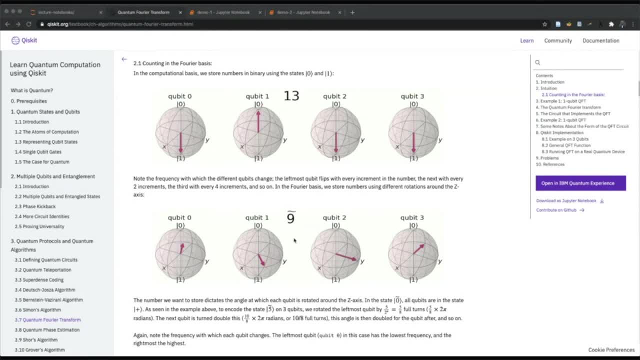 you only have the freedom of being in the up or down state. In this particular case, in the Fourier basis, you can now play with phases on the equatorial plane, And this is exactly what it means to do: a quantum Fourier transform. To go from this picture at the very top: 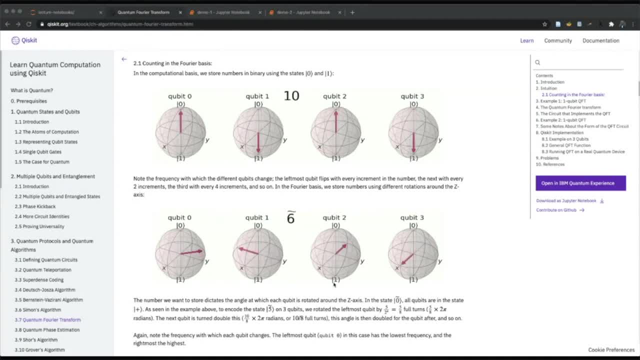 to this picture at the very bottom. So let's take a break now and we'll go through in some detail how exactly the quantum Fourier transform works.